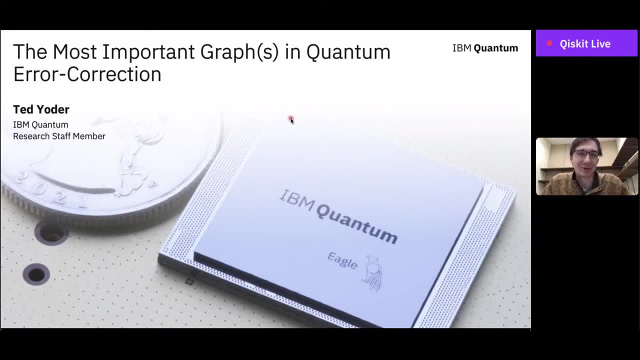 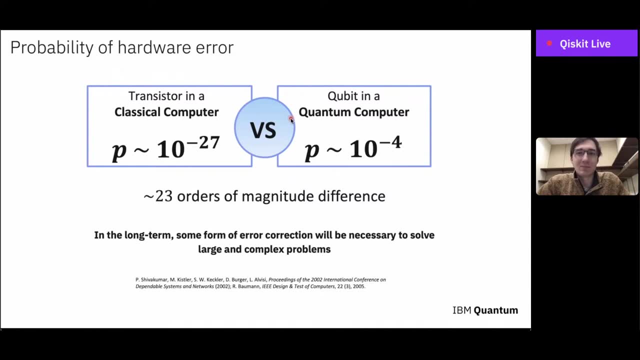 a few most important graphs in quantum error correction. So let's get started here. So the main problem with our quantum computers nowadays is that the error rates are too high. If we compare to transistors in classical computers, with our qubits in quantum computers, we have about 23. 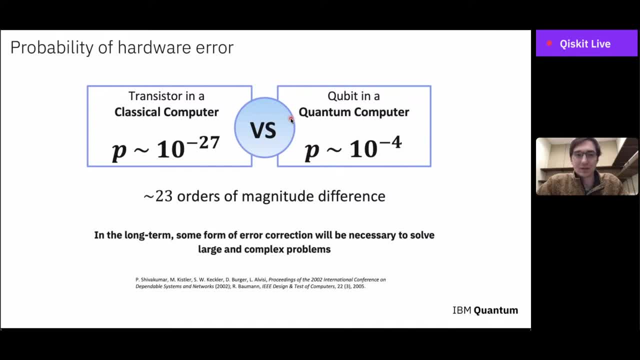 orders of magnitude difference in the error rates. So this really makes the point that we need in the long term, some sort of error correction to solve large and complex problems, Because right now, even if you do have error rates of 10 to the minus 4,. 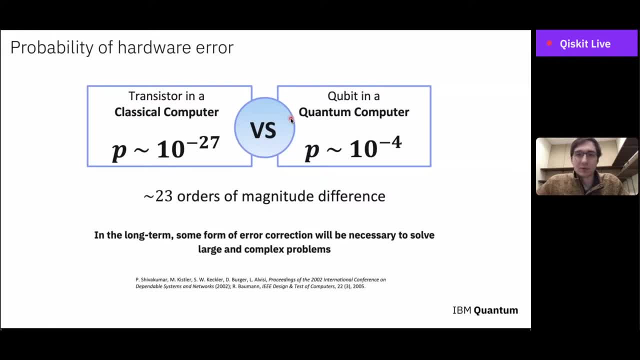 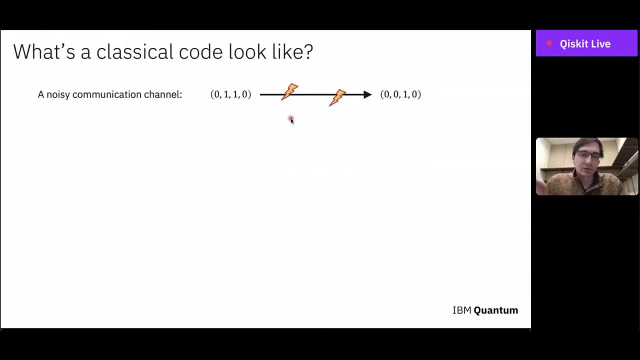 you're only running circuits of like 10,000 gates before the error rates become unmanageable. So this talk is going to be focusing on quantum error correction. but what actually does classical error correction look like, So we can take some inspiration from that? So in the classical case, 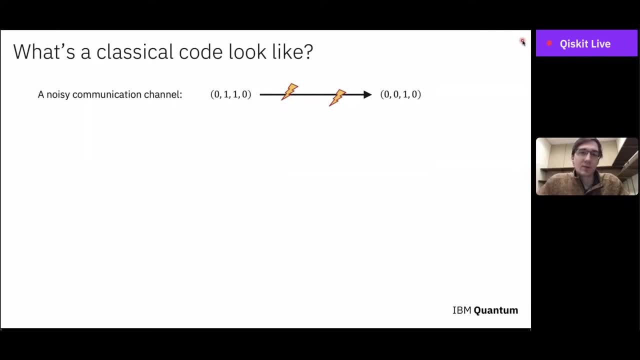 maybe Alice wants to. She sometimes sends Alice to send Bob some bit string. So here: 0, 1, 1, 0.. But there's some noise in between, There's a noisy communication channel and when Bob gets it the message is corrupted. So I think often when people look at this scenario, 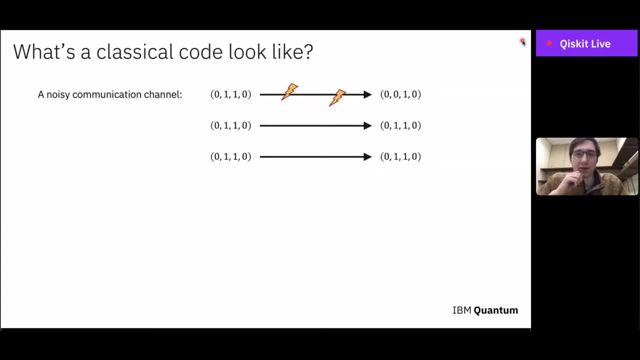 and give some example of a classical error correction code. they talk about the repetition code. They say, well, Alice could just send the same message three times and then hopefully Bob gets it, But the representation here isn't very powerful. So he, it looks Terre İ, and how these xも. 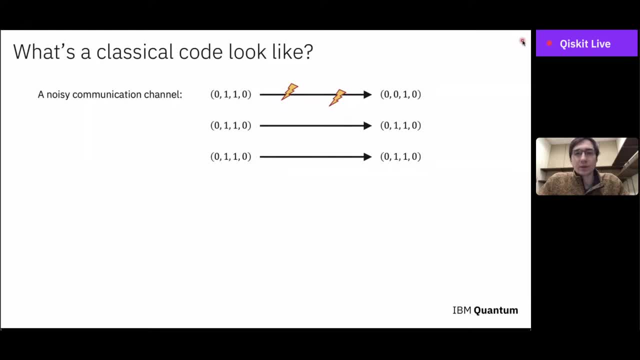 gets it and can majority vote on the bits that he receives in order to decode the message. So this works. This is a valid classical error correcting code, But the sort of implication here is that you need to copy the message that you're sending. 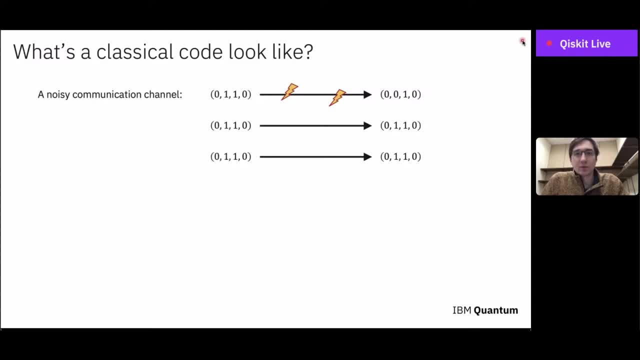 which is something we don't like to do in quantum computing because of the no-cloning theorem. So there's actually a different perspective of classical error correction that I want to drive home here, And to do that we'll use this example of the 7-4-3 Hamming code. 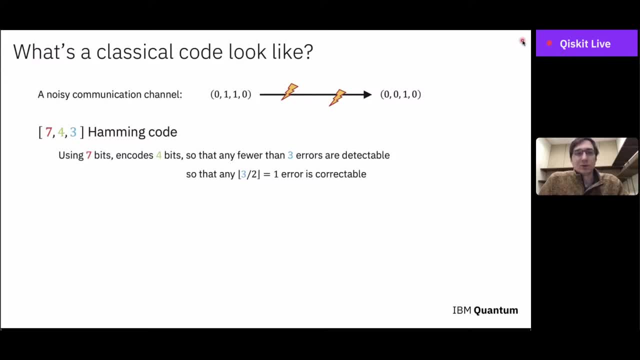 So what do these numbers mean? Well, the 7 means that you're using seven bits, The 4 means that you're encoding four bits, four logical bits, And the 3 means that you can detect any fewer than three errors. So you can detect one error or two errors. 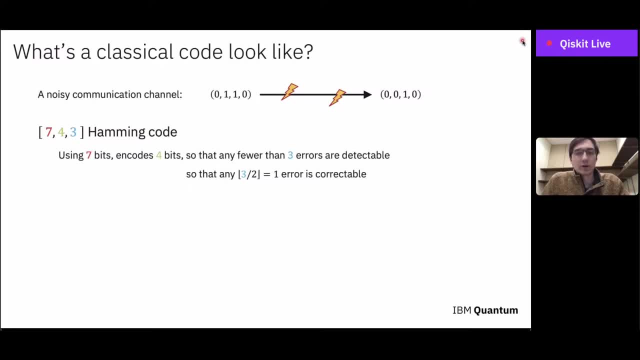 Or, alternatively, that you can correct any one error, which is like 3 divided by 2, and then you take the 4 of that. So here's what the 7-4-3 Hamming code looks like. 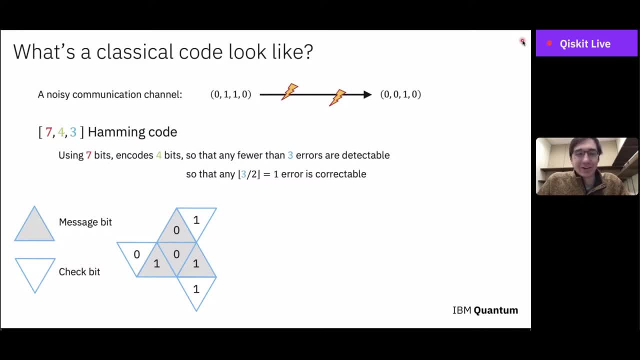 And you'll learn as I go through this talk that in error correction we like to draw pictures a lot. So here's my picture of the 7-4-3 Hamming code. So every triangle here represents a bit, And Alice is going to send all the bits. 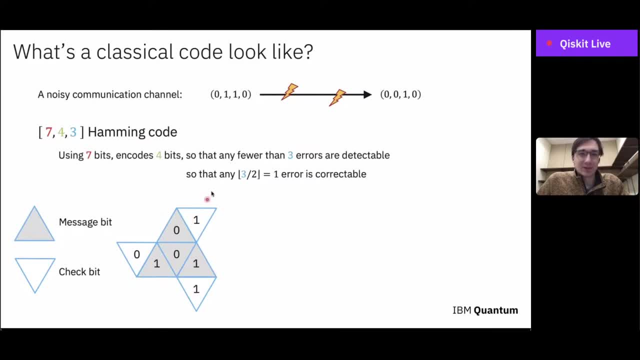 All seven bits to Bob now. So she's encoding her four bits and seven bits. The gray bits are the actual message she wants to send, so 0110.. And then the white bits are extra check bits to do the error correction. So the parity checks are the important thing. 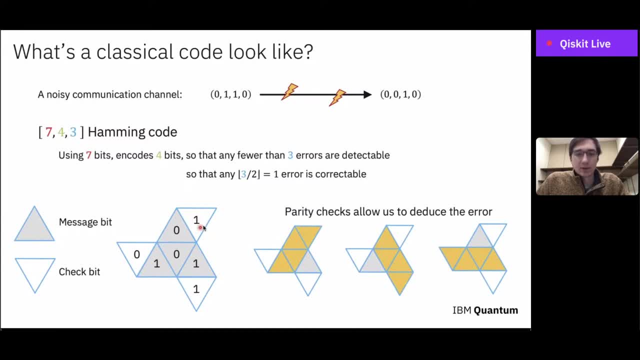 So the way that we set these check bits is by making sure that the parity along these lines is equal to 0 mod 2.. So if we add up the bits along any of these lines indicated in yellow over here, you get 0 mod 2.. 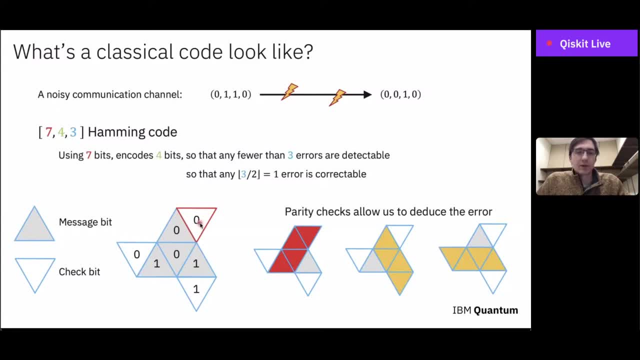 So that when an error occurs, such as an error on this check bit, you'll see that some of the parity checks light up- In this case, just the one parity check lights up- And Bob, when he gets all seven of these bits, can tell that, oh, most likely this is the 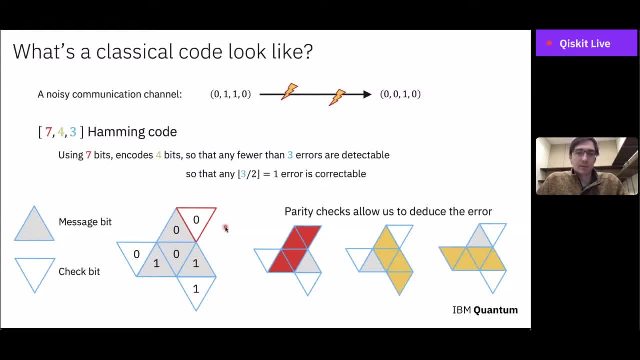 bit that was flipped, the check bit. But let's say that one of the message bits flips, then both of these checks light up, So Bob can tell that this is the bit that flipped. And then, if the middle bit flips, all three of the checks light up. 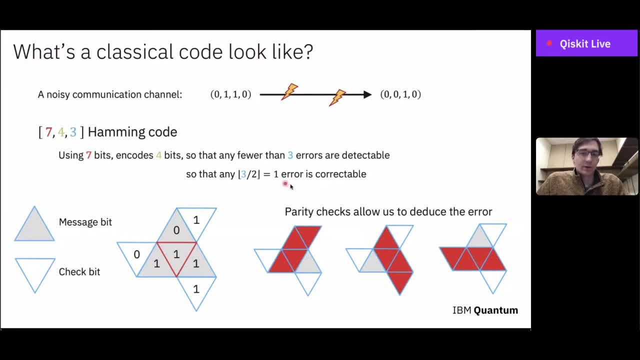 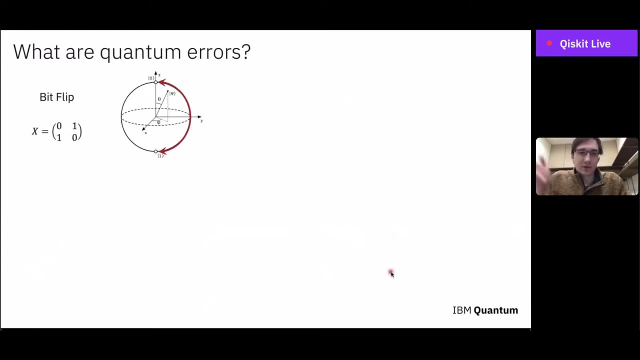 So this is why one error is correctable. You can see that putting one error anywhere leads to a unique syndrome, A unique combination of parity checks that fires. I hope that makes sense And of course, you can ask any questions in the chat as we go along. 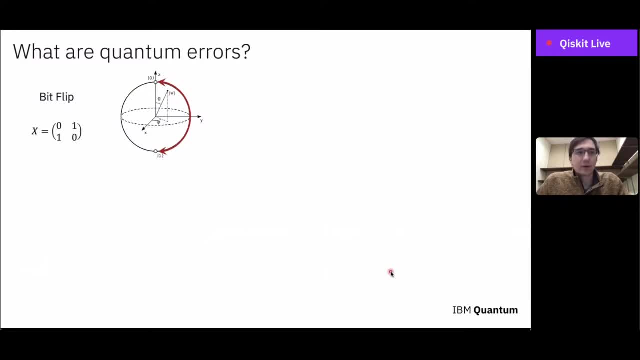 So that was the classical case. In the quantum case there's another wrinkle: is that the quantum errors are a bit different than classical errors, So of course we have bit flip errors, like we were talking about in that classical case. 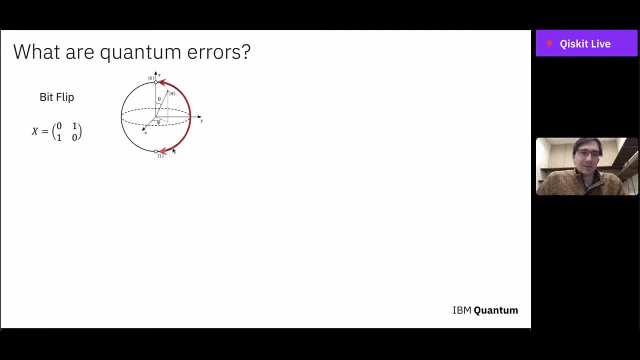 This is the Bloch sphere, by the way, Hopefully, Hopefully, you're familiar with this. The pure states of a qubit lie on the surface and then the mixed states lie inside And a bit flip takes you from the top to the bottom. 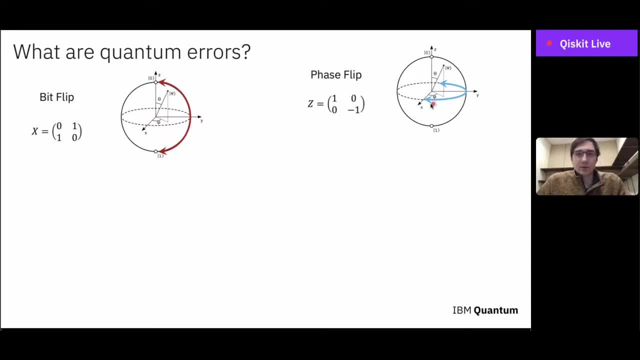 Now there's also phase flips in the quantum case, which take you around the z-axis, And there's bit plus phase flips, which, well, is a combination of the bit flip and the phase flip, And sometimes it's the same thing. 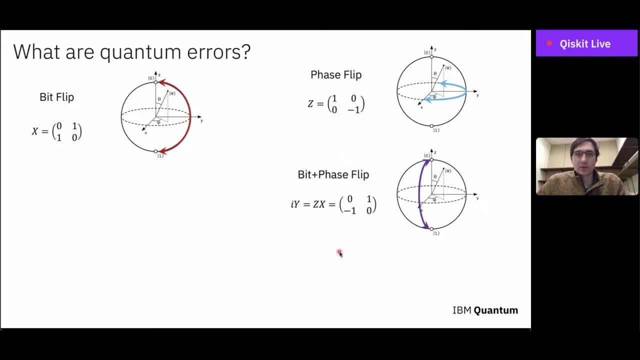 But the bit flips are all made by x, z and y falling matrices, And so all of these sort of form a basis of quantum errors, Whereas in the classical case we just have the bit flips. So you might think that quantum errors can be somewhat analog. because we're on this, 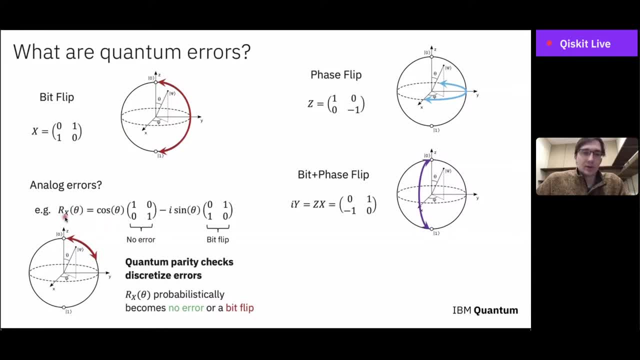 continuous surface And maybe there's a small error, like this rotation, where theta could be really small, and maybe that error is like hard to correct because it's so small. but a key point of quantum error correction is that when we measure quantum parity checks. 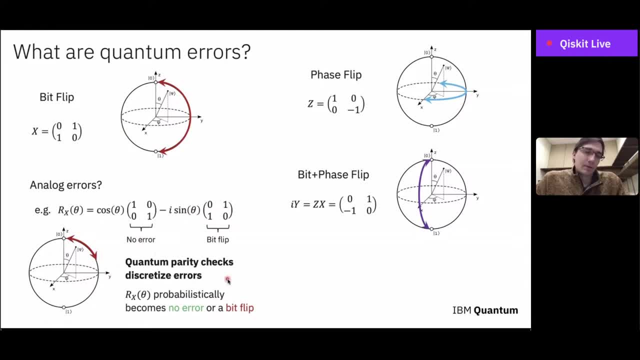 which I'll explain, I think, on the next slide. when we measure those parity checks, we disparatize errors, so we sort of project this, what this, this analog error, this sort of continuous, continuously parameterized error into some combination of no error and a bit flip error. 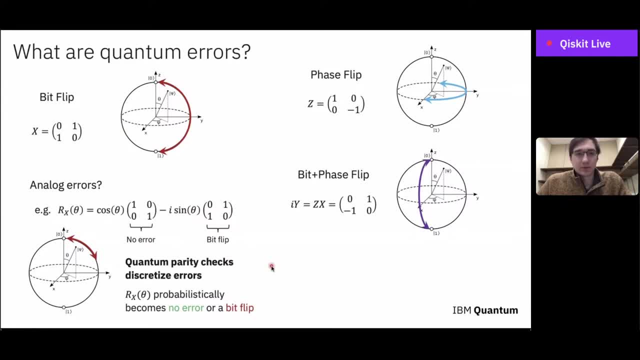 and then the bit flip error should hopefully be correctable because we're using a quantum error correcting code that can correct that. yeah, so then, the last thing I want to point out is just that these poly matrices anti-commute, and this is sort of the principle that we're going to use to detect errors using quantum parity checks. 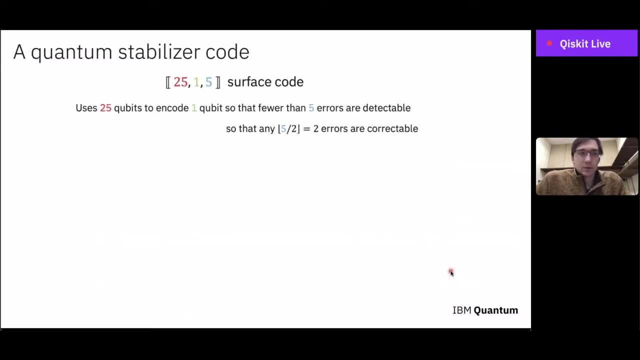 so let's see how that goes. so when we, when we talk about quantum parity checks, really this is the, this quantum stabilizer code formalism. so here's an exemplary quantum stabilizer. the stabilizer stabilizer is equal parity checks. that's what you need to know. 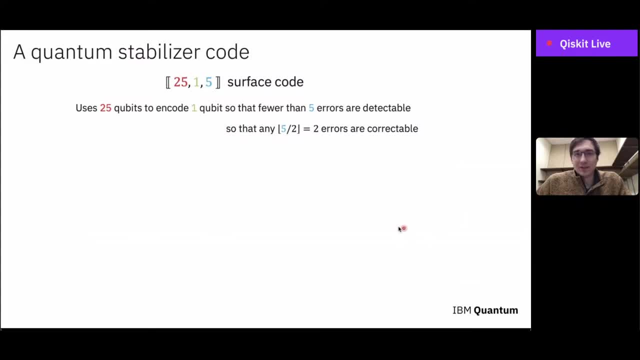 so here's a 2515 quantum service code, and it's quantum because we use the. we now use a double bracket instead of a single bracket, like like for the classical code. so we use 25 qubits to encode one logical qubit and we can detect any fewer than five errors. you. 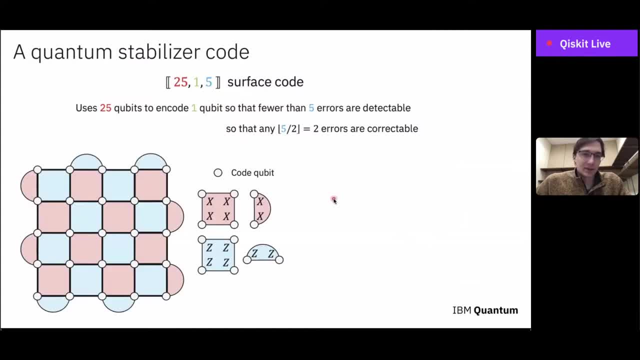 can also correct any two errors. so it looks like this: where the in in red we have X type parity checks and in blue we have Z type parity checks. so essentially the parity checks are operators that you measure and we'll. we'll show later circuits and how you actually measure these, but when you get zero, that indicates no error. that 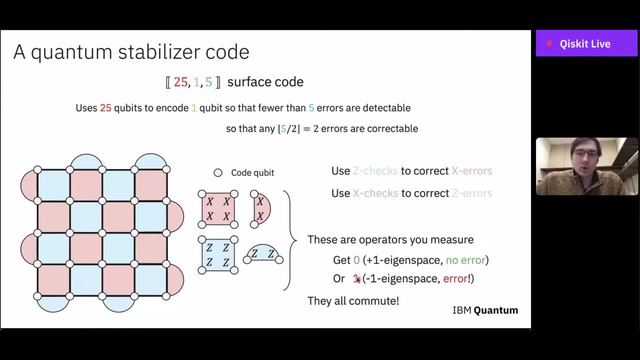 you're in the code space and if you get one from your, your measurement, then it indicates that there was some error and it's, it's the job of a decoder, a decoder or decoding output algorithm, uh- to figure out where that error occurred. um, notably here, all the parity checks. 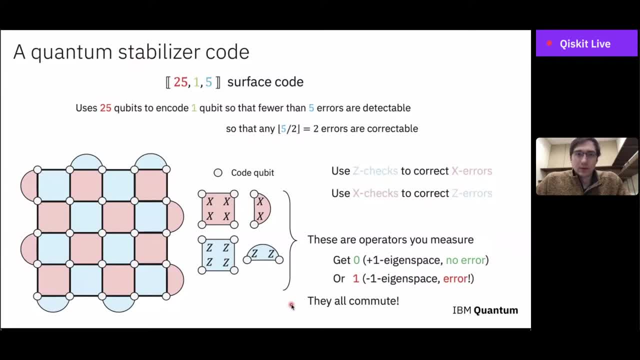 commute. so that means in, in quantum language, that you can. you can simultaneously deduce the, the eigenvalues of all of these parity checks, and then, uh, the. the last thing I want to point out is that you use, uh the Z checks to correct the X errors and the. 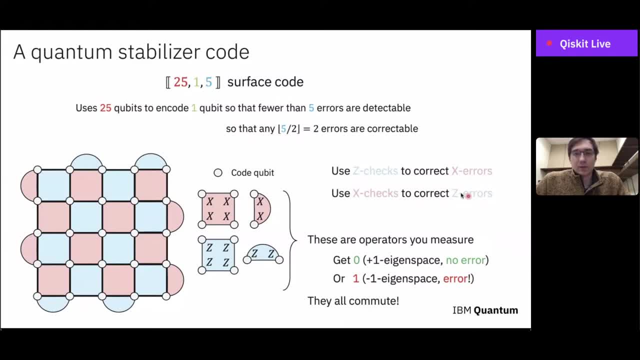 checks to correct z-errors. I could have also written detect x-errors and detect z-errors, And essentially the reason why that works is because of this anti-commutation property from the previous slide. So let's look at some examples. So if there's an x-error here, 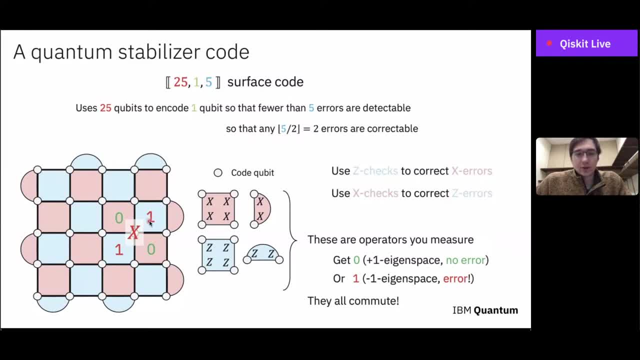 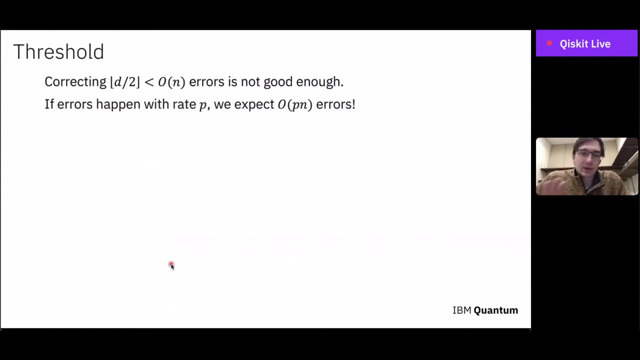 then it anti-commutes with these adjacent z-checks, And so those indicate an error. Those have value 1 when you measure them, And similarly, if you have a z-error here, the adjacent x-checks indicate an error. Okay, And here I'm getting. 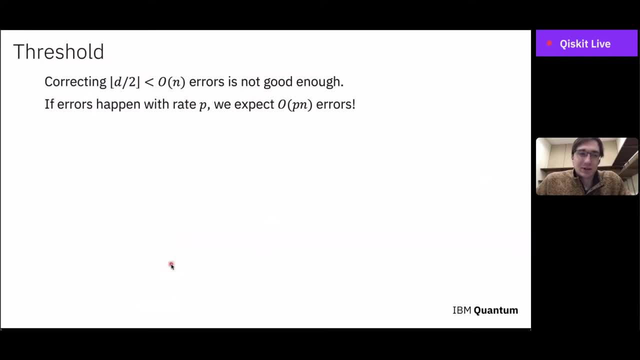 Yeah, Here I'm trying to make the point that correcting So for the surface code when you scale it up. the code distance d which, remember, indicates how many errors you can correct: d over 2 errors you can correct if that's fewer than the number of physical qubits that you're using. 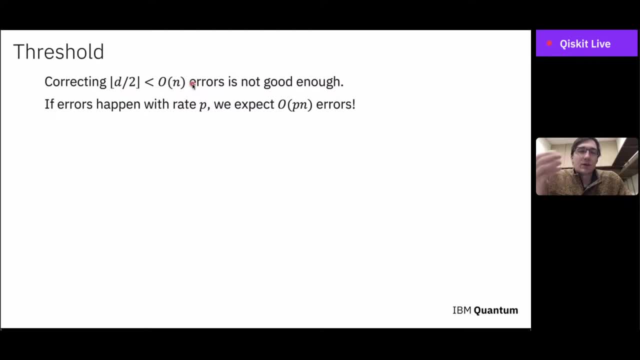 then that's not always going to be good enough. So what you really want is that if errors are happening on your code, some rate p, then you expect order p? n errors and hopefully you should be able to correct that which the distance argument alone is insufficient to handle. 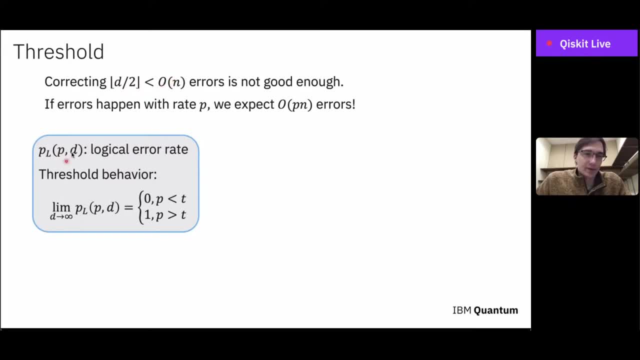 So let's define this logical error rate, which This is the logical error rate in this model where errors are happening with rate p, Then we can. Then we can decide whether this function p sub l has a threshold behavior or not. 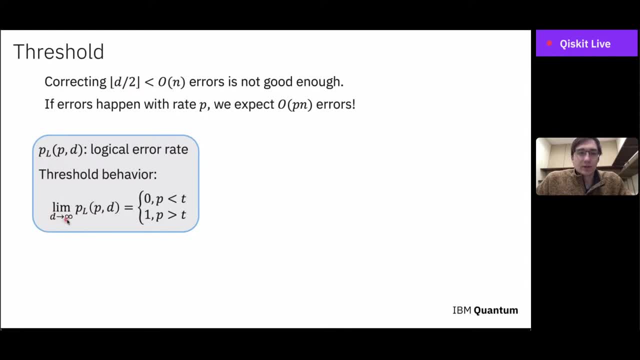 So, as we scale up the code, the distance goes to infinity. Does this function go to zero, As Does it go to zero at least for some values of p, Or does it go to 1?? So, if it has this behavior where there's like a step, 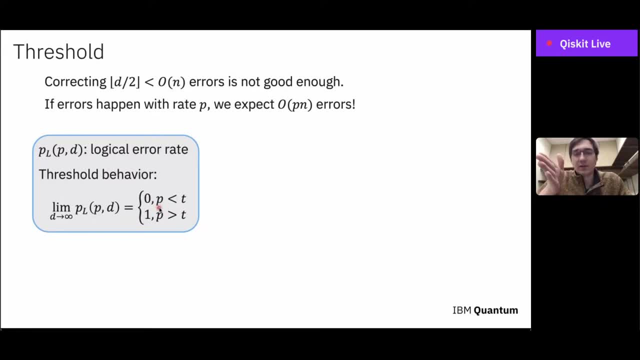 where if you're below the threshold t, then your error rate goes to zero, and if you're above that it goes to 1, then we say that the code has a threshold. Yeah, so t is called the error threshold, and then this threshold depends on. 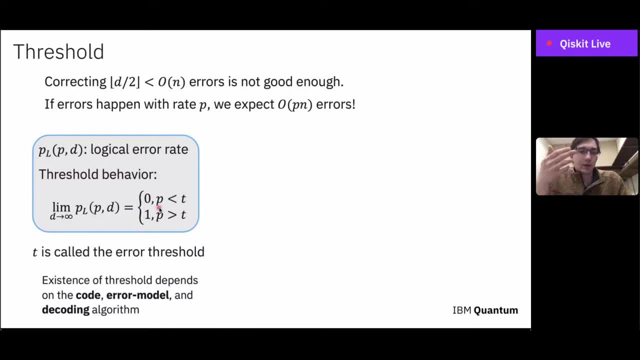 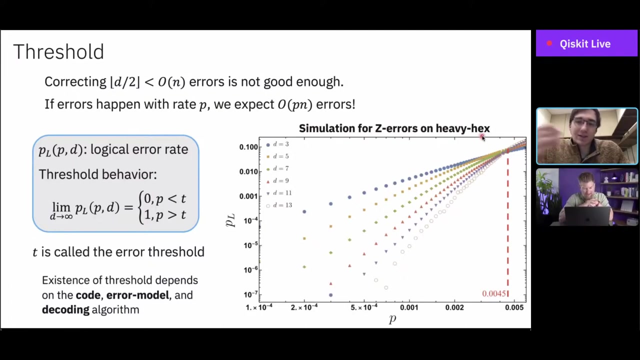 the code that you're using, also the error model, also what decoding algorithm that you're using. So, for instance, here is a: This is a plot for this. Z error is occurring with rate p on the heavy hex code, which I'm going to get to next. 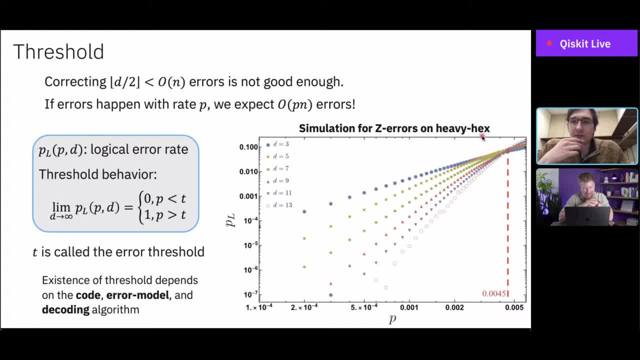 But in this case it's roughly the same as the service code. Sorry to bother you, Todd. I was wondering if you could clarify what the distance of the code is. I think there was some Right Right, Right Right. 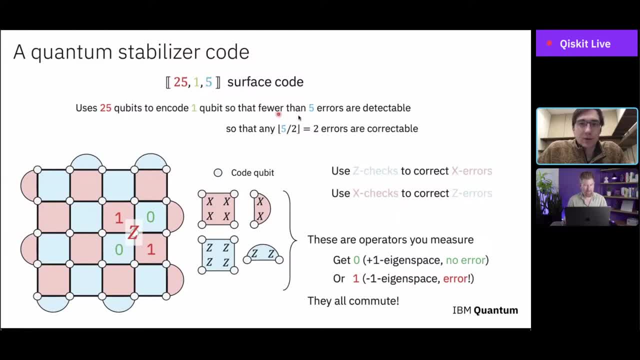 really is just a measure of how many errors are detectable or correctable. So if you have fewer than D errors, then it's detectable, And if you have D over two and then you take the four. So if you have fewer than D over two errors. 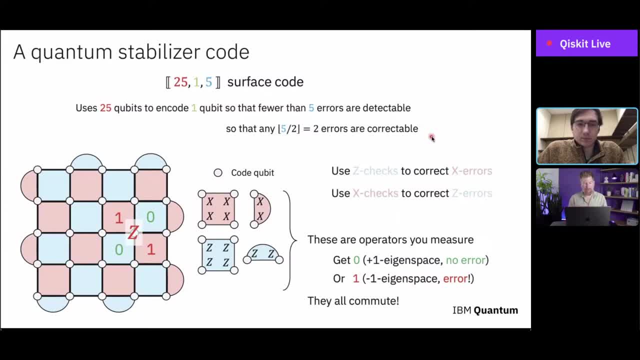 then they're correctable, right, Right, and I might add that I think of this as being a physical thing, as like how many qubits like physical qubits? do you need to implement a logical error corrected? one as well, And that depends. 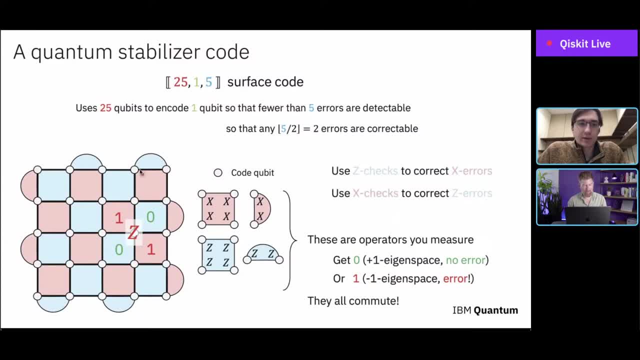 Yeah, so you can also think of this as: how many physical qubits do you need to act on to do a logical bit flip or a logical phase flip? All right, thanks for the clarification. Yeah Right, so we were talking about this threshold. 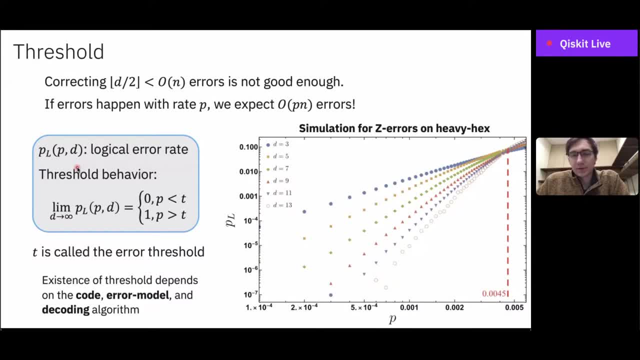 So here's a plot Of the logical error rate versus the physical error rate for a particular code, which I'll explain later. And you can see this behavior where, below this point, where all the curves cross, you're getting lower logical error rate as you increase the distance, as you increase the code size. 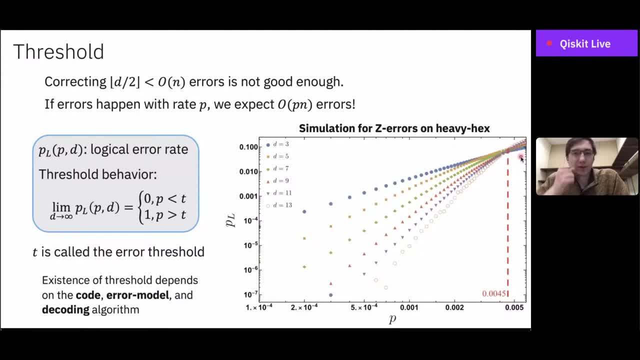 And then, above that point, you're getting higher logical error rate. So this is emblematic of the threshold error, the threshold error rate. So this is the most. this is the first, most important graph, or you know, not just specifically this graph. 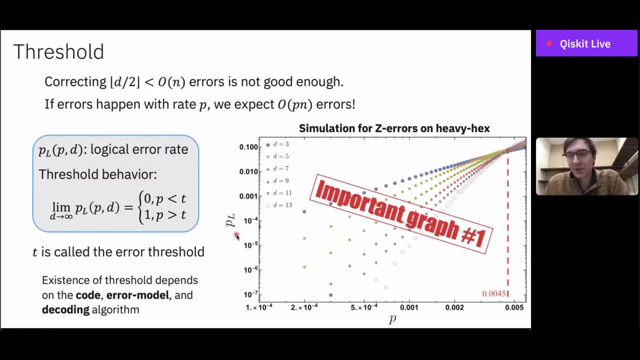 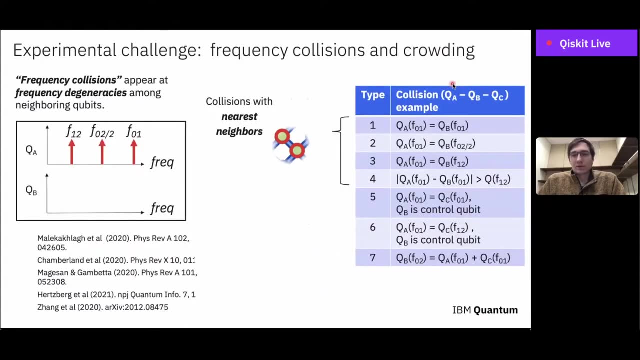 but the fact that you can plot logical error rate versus physical error rate and then you can see a threshold sometimes, And I think this was also said in Nick's quiz kit tutorial. Okay, so now I'm gonna move on. So I'm gonna move on. 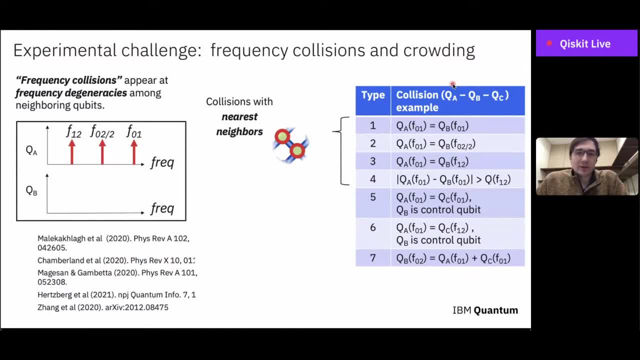 To essentially the second part of the talk where I described our heavy hex code. So one of the challenges we face in experiments with our qubits at IBM is that they have fixed frequencies And if the frequencies of qubits next to each other in the lattice line up in certain ways. 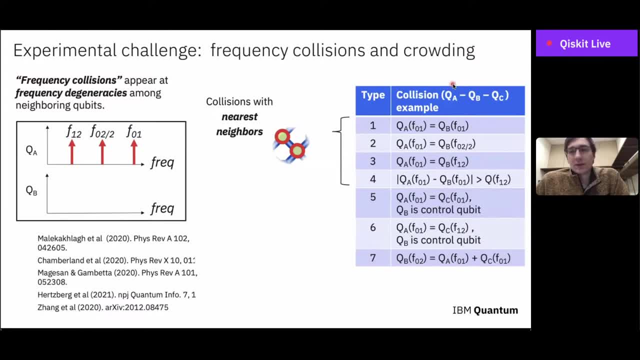 so they have certain frequency degenerations. then when you do our CNOT gates, the CNOT gates will have a lot of error. So what are some of these degeneracies? Well, if the neighboring qubits have the same transition frequency between their zero and one levels, 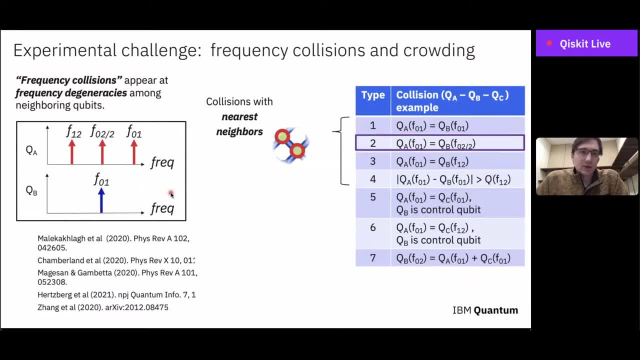 then you get a frequency correction. Or if the transition between zero and one of the target qubit is like the transition frequency between zero and two divided by two of the control qubit, then you also have a collision. So there are a lot of these conditions. 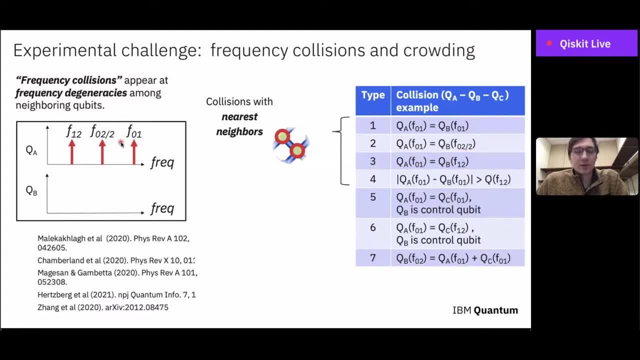 and I'm not going to go through each one, but essentially you want to avoid these by setting the frequencies appropriately, if possible. Now there are also collisions, even between next nearest neighbors in the lattice, And so these are things that you also want to avoid. 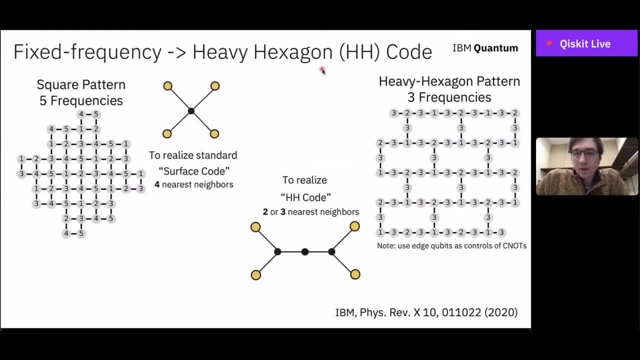 So that leads us to the experimental layout of qubits that we actually have at IBM. So on the left there's the square pattern of frequencies, which is something that you would use to implement, like the surface code which I showed earlier. So in this case every qubit has four nearest neighbors. 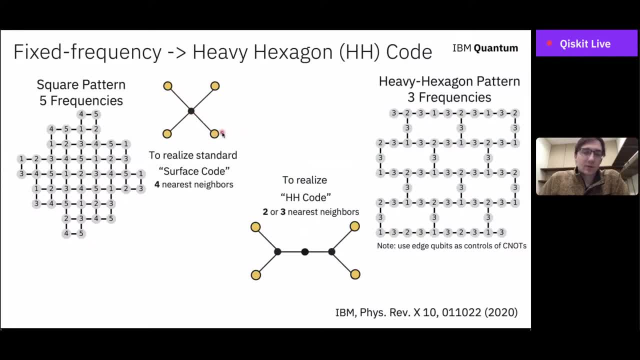 and what that means in terms of the frequency collisions that I showed you on the previous slide is that you actually need five frequencies to avoid those collisions. Now, in contrast, if we look on the right here, this is the heavy hexagon lattice. 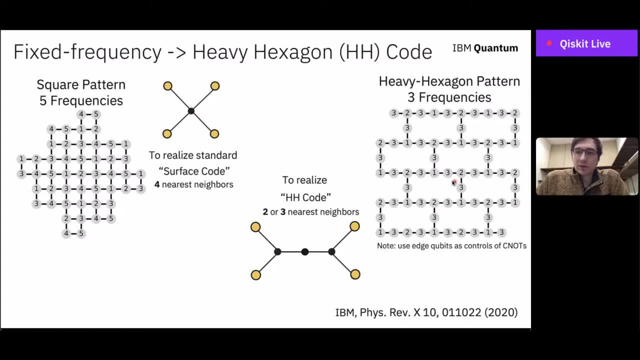 So here you can think of each of these cells as a hexagon, with qubits on the vertices and the edges. So this is the hexagon with qubits on the vertices and the edges of the hexagon, And here every qubit has either degree or three. 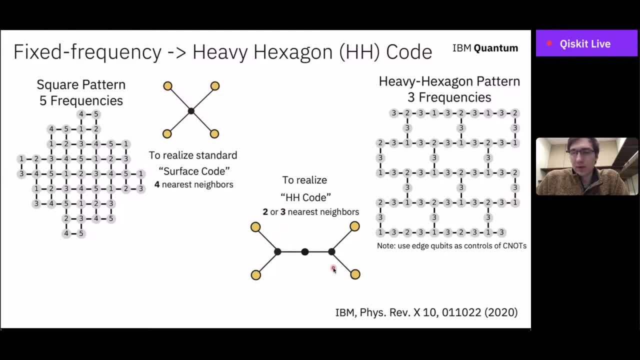 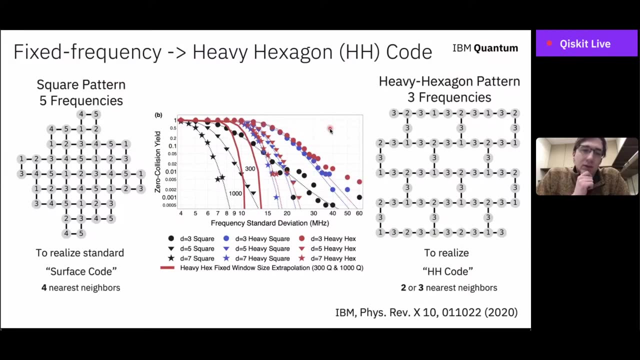 two or three. So two nearest neighbors are three And you actually only need three frequencies to avoid the collisions. So that's a big advantage And we can quantify this by looking at something called the yield. So when you actually fabricate the qubit, 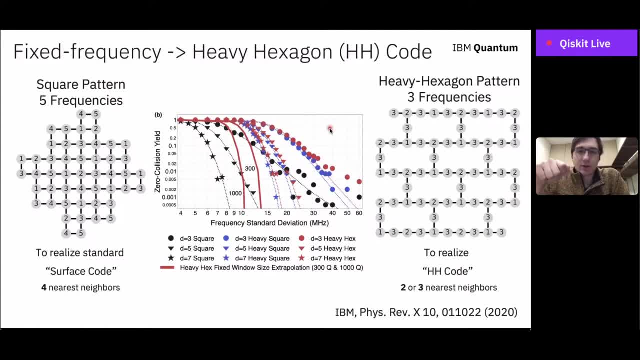 there's some standard deviation in the frequencies of the qubits. Although you try to set them to some value, those deviate, So you can end up with frequency collisions anyway, even when you're trying to set the frequencies to the one, two, three values over here. 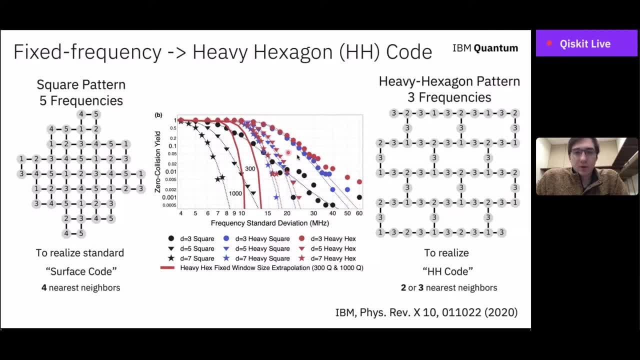 So what this plot is is trying to communicate is that if you use the heavy hex layout instead of the square layout, you end up with fewer frequency collisions. You end up with greater yield. So you can see that the red points are higher than the black points. 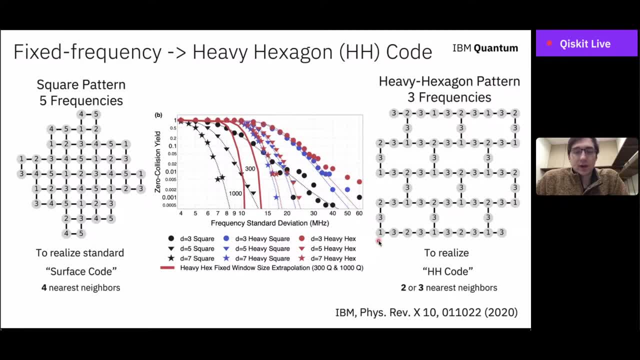 The black points indicating the square lattice and the red points indicating the heavy hex. And around 20 megahertz standard deviation is what we have currently in our FAB. So this heavy hexagonal lattice is great for avoiding frequency collisions and increasing our yield. 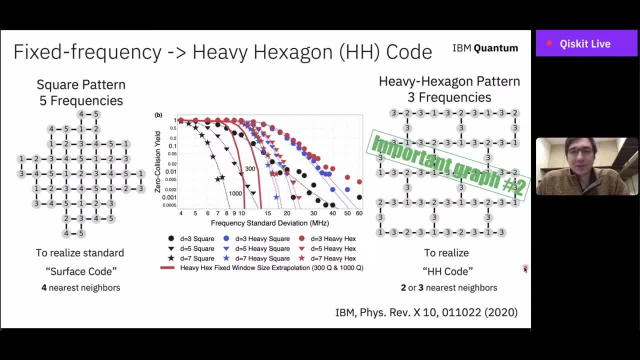 So I'm going to indicate this as important. graph number two: This is a graph in the mathematical graph theory sense that there are nodes, there are vertices and edges, and this is very important, Not just specifically this graph, I guess, but the connectivity graph. 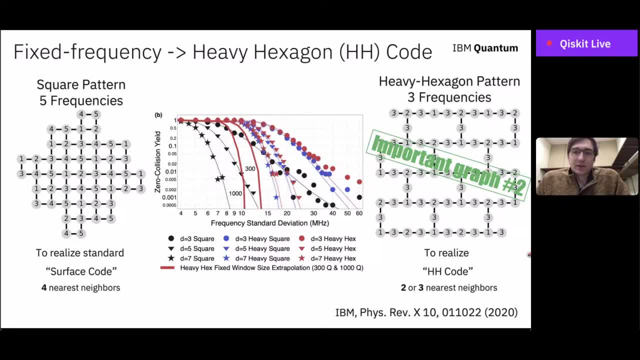 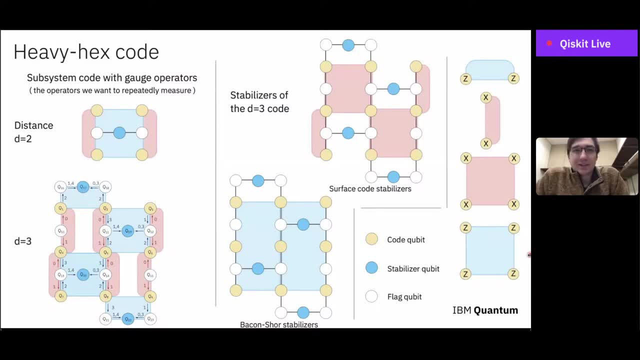 is very important for determining what error correcting code you can actually implement. Okay, so what error correcting code do we actually implement? This is the heavy hex code. Okay, so there's a lot going on here, but essentially there are parity checks that we measure. 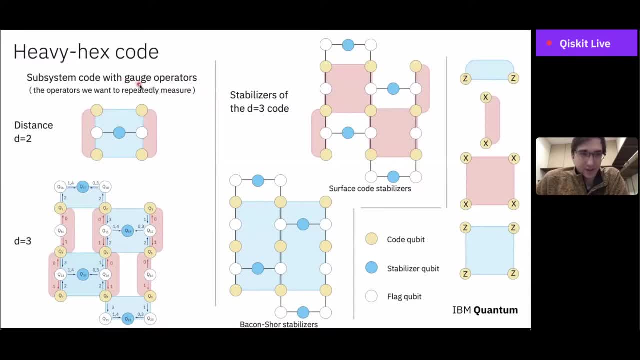 Here I call them gauge operators because it's a technical term. but so there's X and Z type parity checks. These are supported on the code qubits in yellow. so here the distance to code has four code qubits and the distance through the code qubit has four code qubits. 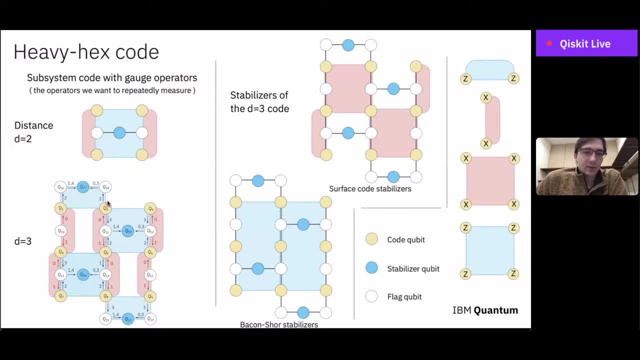 Every code has nine code qubits- yellow- Okay, so the gauge operators are what you measure. Now, this code is a bit different than the surface code that I showed earlier, in that, once you go to distance, three at least these gauge operators- 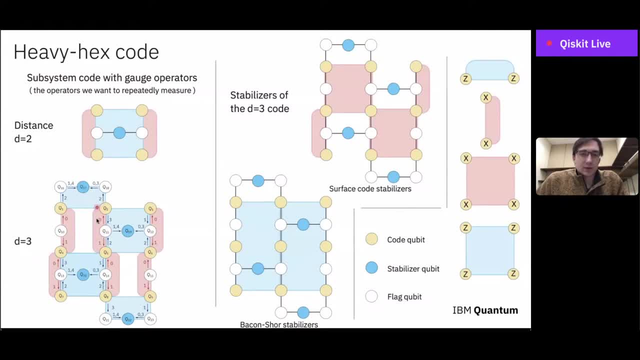 don't all commute. So, for instance, this guy is X- X on these two code qubits and this guy is X- X on these two code qubits. and this guy is X- X on these two code qubits, So they would anti-commute here. This means that the useful information you get from these 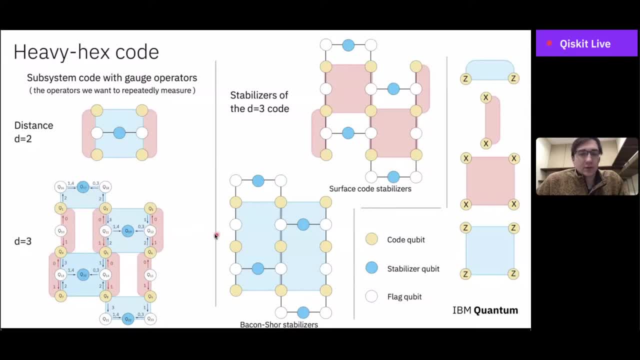 gauge measurements is actually only certain products of the gauge operators, and those products of the gauge operators are the stabilizers. So that's in this center panel. I show you the stabilizers of the distance, three heavy hex code Right. so the X type. 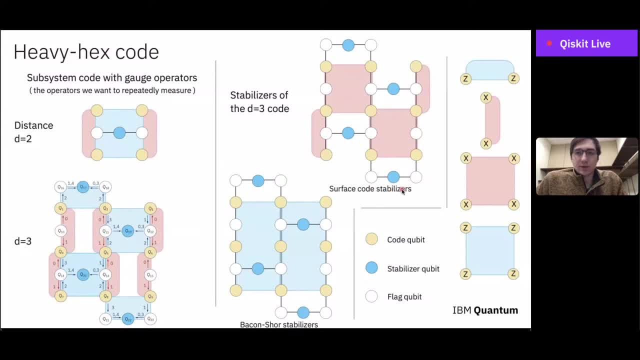 stabilizers actually look like the surface code stabilizers. There are some weight four guys and weight two guys on the boundaries, and the Z type stabilizers are actually these long strips, so they're weight six. They act on six code qubits- those six- and 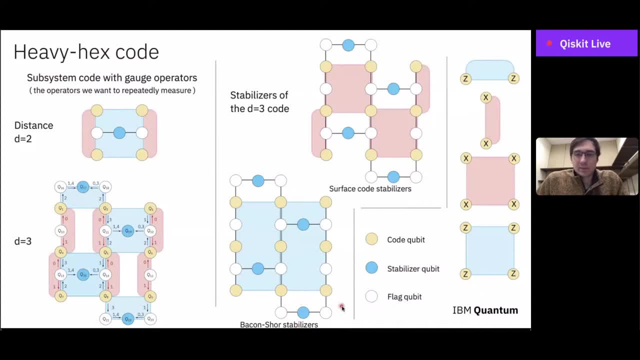 they're what we call Bacon-Shore type stabilizers. Okay, so I explained the code: qubits in yellow and then the. the other two colors of qubits are just used for the readouts of these parity checks. So I'm going to show some circuits next. 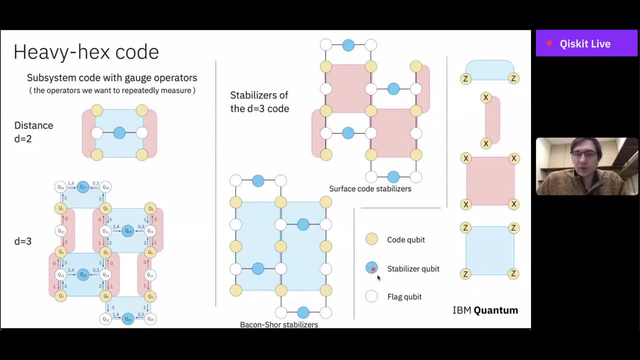 and so when you measure these helper qubits, the stabilizer qubit and the flag qubit, you'll learn these parity checks, You'll learn the values of these parity checks and hopefully that'll give you enough information to correct the error. 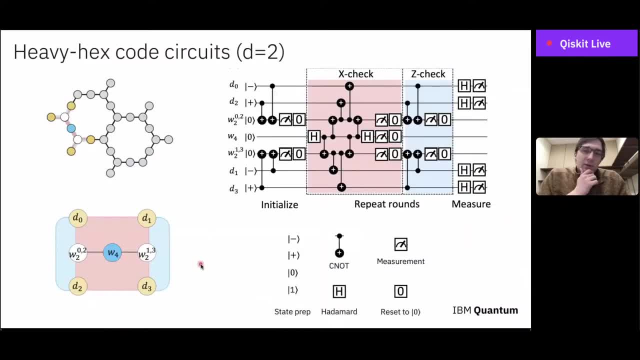 So how does that go? So here I'm just going to talk about the D equals two code. So you can see that this D equals two code is like a unit cell of the D equals three code. and then you just combine these unit cells, you translate them around the lattice to make larger. 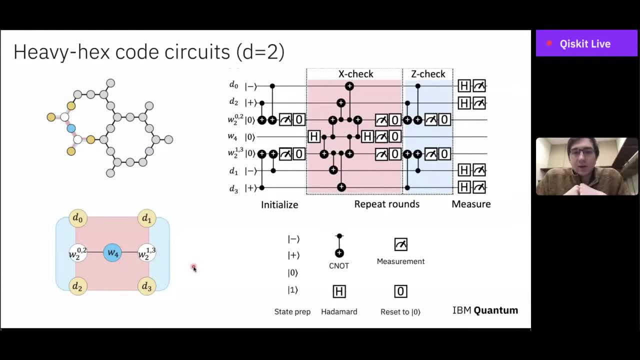 and larger codes. So if we just look at this, we get a good idea of how the larger code works as well. Right, so this is the code and you can see it laid out here explicitly on the heavy hex lattice. And here's the circuit that we use for error correction. 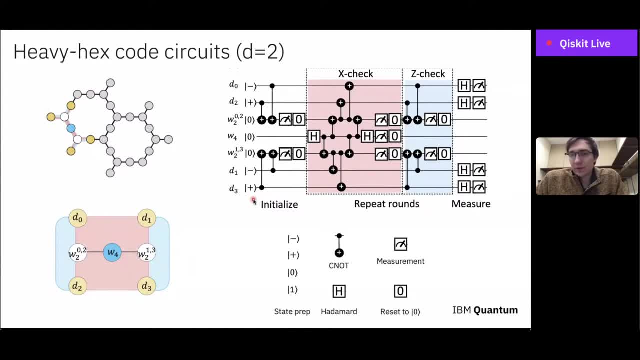 and I think this is also what Nick Braun does in his tutorial, Or actually maybe he prepares it differently, but this is what we do in our experiments in there For our paper. So we prepare all qubits in a product state to start with, So each is in just. 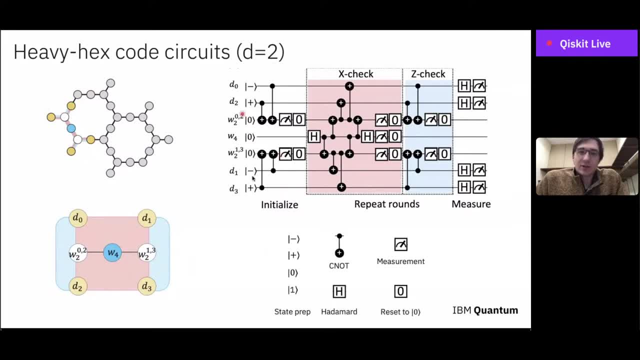 its individual single qubit state and then we project into the code space. That's this initialized step. So this initialized step is actually the same as the z-check step. So it's measuring the z-type stabilizers, And the way it does that is by reading out the eigenvalue into these helper qubits here. 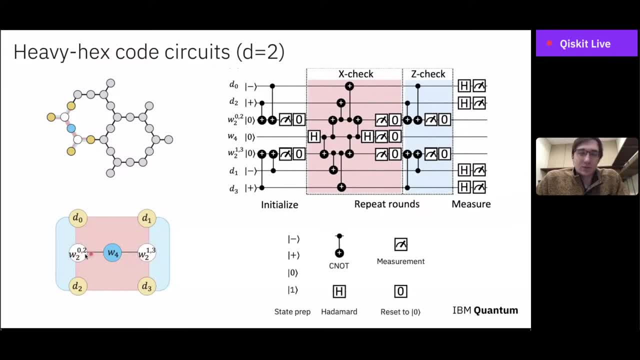 which I guess I'm just indicating w2 for weight, two qubits. And then what we do in our experiments is we repeat the parity check measurements many times. So you measure the x-check and then the z-check, and this block is repeated. So you measure the x-check and then the z-check, and this block is repeated. 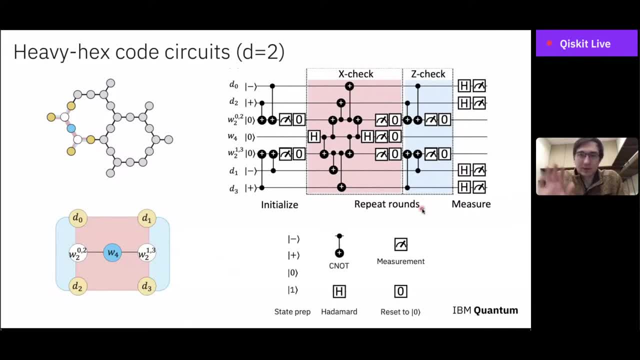 And on the next couple of slides I'll explain why this circuit works, But for now just take this as granted. And then at the end we measure out all the qubits. And so this is how we read out the logical information, After it's been protected for some number of time: steps here in the middle. 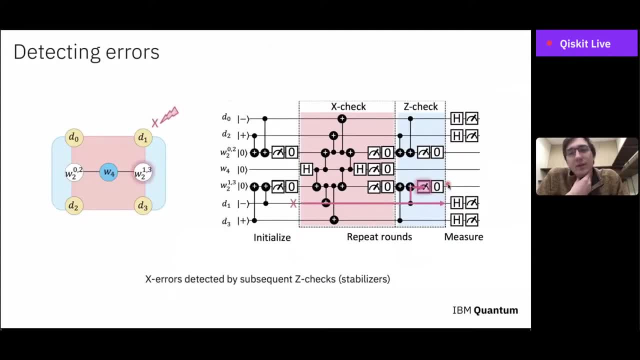 Okay. So why is it so important? Yeah, That's a very important part of this task. so why does the circuit allow us to detect errors? So let's say that an X error occurs here on this data qubit one, Then it passes straight through the X check. So the CNOTs. 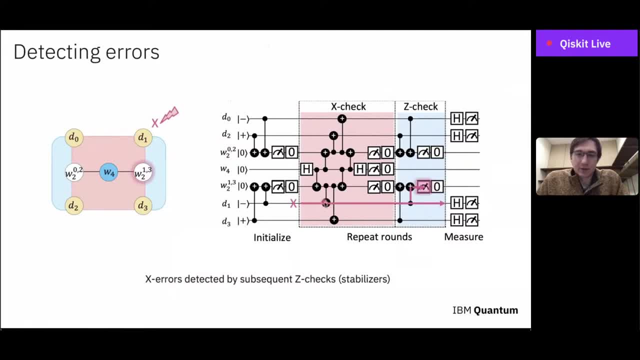 you know, if the target qubit of a CNOT is flipped, that doesn't change the control qubit of the CNOT at all, So it passes straight through the X check. But then when we hit the Z check, the X error propagates up to the measurement And so we see that X error. So the Z check ends up. 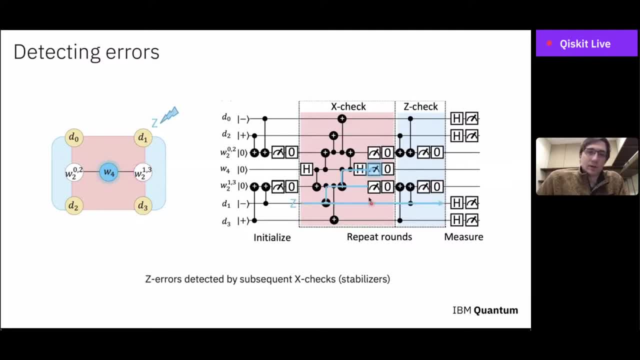 detecting the X error. Likewise, if we have a Z error, it passes straight through the Z check. But for the X check it passes straight through the X check. But for the X check it propagates up to the X stabilizer measurement, And so we detect it there. 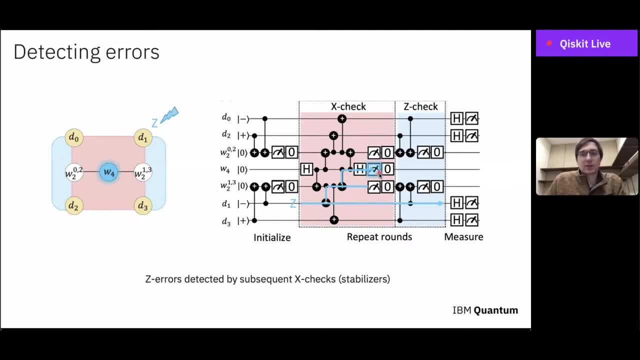 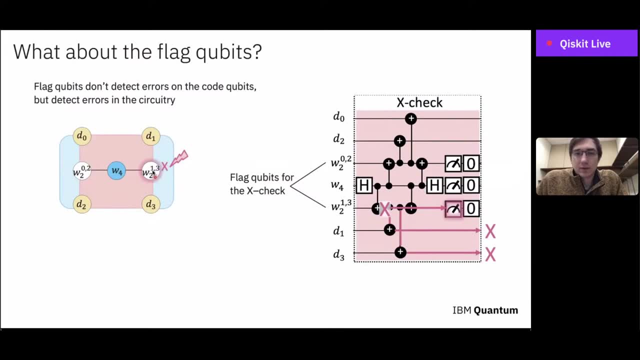 Okay, so the X checks are detecting Z errors and the Z checks are detecting X errors, just as we want. But what happens with the flag qubits? So these are the qubits here- W2 qubits- that are in play when we're measuring an X check, But they actually didn't. 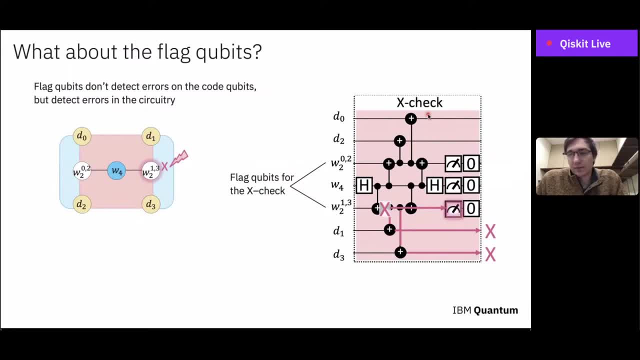 help us detect Z errors at all. They sort of you know they always reported zero when there was a Z error, on the data at least. So actually what these flag qubits do is they detect errors in the circuitry. So in quantum we can have errors both on the data qubits but also. 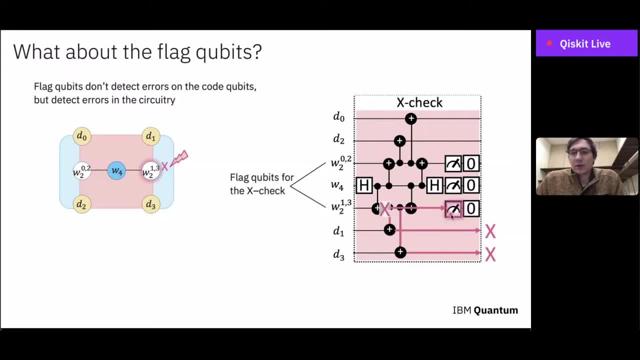 on the other qubits as we're measuring, the parity checks. So let's say we have an X error here. So if we have this error on one of the flag qubits and then scarpe that on the same here x, then it propagates both to the measurement and also to two places on the data. 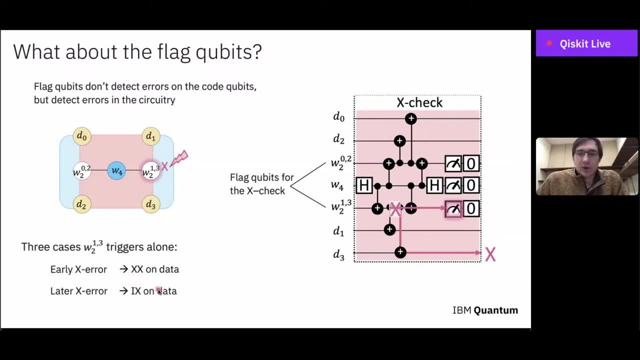 Okay. so if we have this early X error, it propagates to two places on the data. If we have an X error one step later, then it propagates to just one place on the data but also flips the measurement. a very late x error? it just flips the measurement and does not propagate to the data at all. 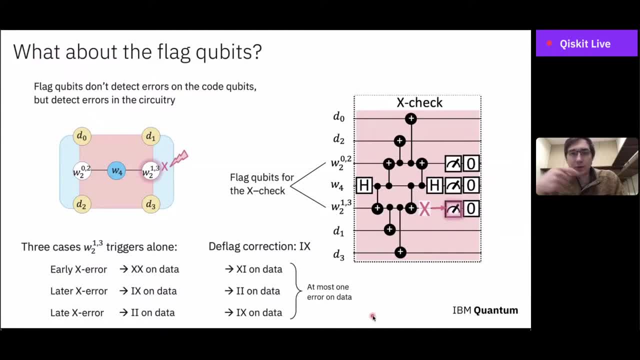 so something you can do to fix this error and use the flag information is, uh, what we call a d flag correction, um. so. so if you see this flag measurement flip and it turns out, if you see this flag measurement flip and not this other one, um, this other flag measurement, so if you just see, 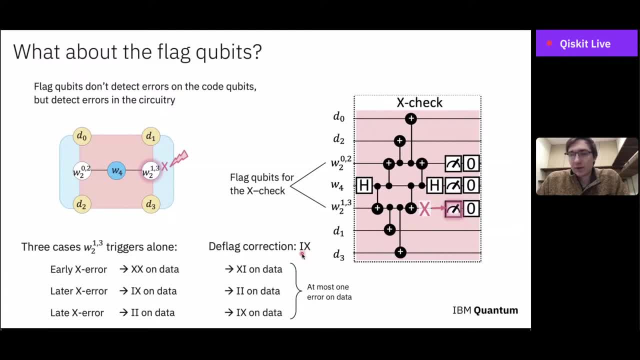 this flag, then what you should do is apply um x to qubit, uh to data, qubit three. so you should apply i x on these, uh on these data tables. and what this succeeds in doing is it transforms these errors that could occur on the data into these errors instead. um, and the important thing about 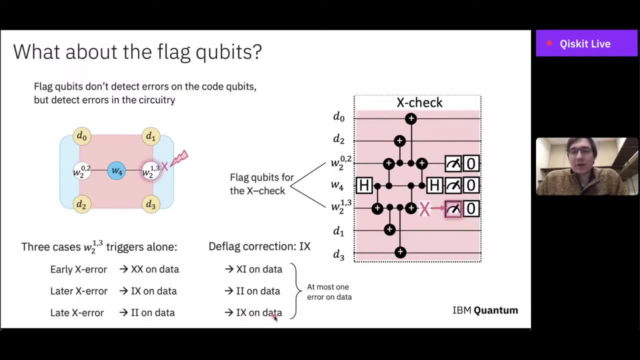 these errors is that there's only at most one error left on the data. so, essentially, if there's one error in the circuit, it propagates to at most one error on the data, and this uh satisfies some definition of fault tolerance, where this, this error on the data. 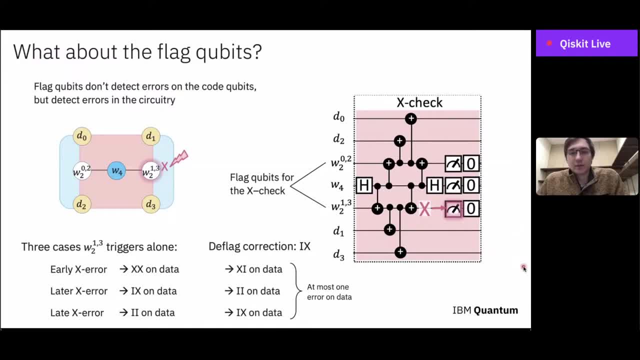 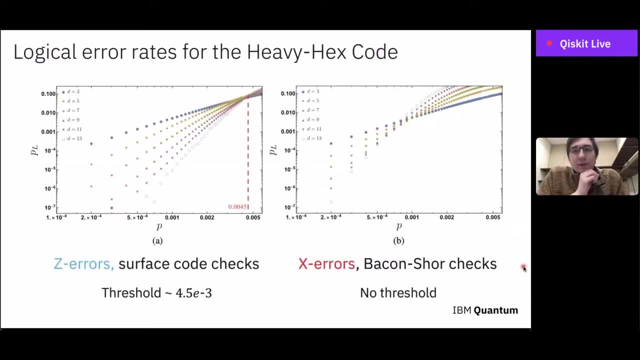 can then, uh, get corrected in later rounds, or at least detected in this case. okay, so, um, those are the circuits and that's how you use the, the flag information and circuit information. uh, so i just want to show the complete set of plots. uh, for the heavy hex code. you saw the one. 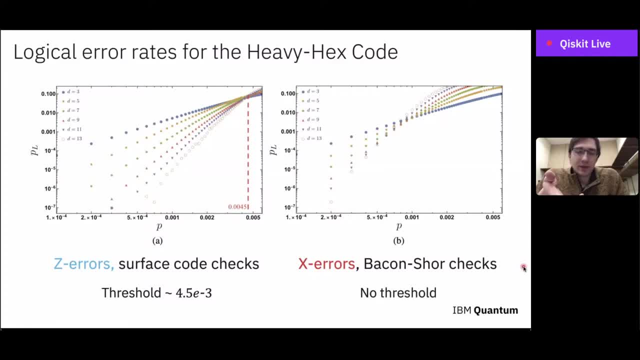 on the left earlier. this is where there's z errors and uh and the surface code checks um. but then on the right we have the uh the case where there are x errors and we're using these bacon shore type checks. now the thing about the, the bacon short type checks is that there's 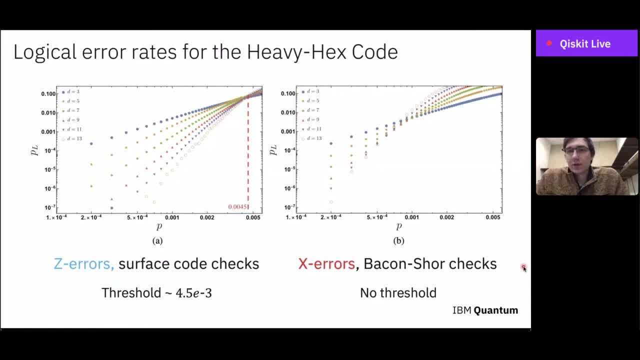 no threshold um. so, like whatever decoding algorithm you use, uh, there's. there's no like asymptotic threshold um, but you can still see uh that if your, if your physical error rate is is low enough, at least for these finite size cases, you are getting some improvement uh, as. 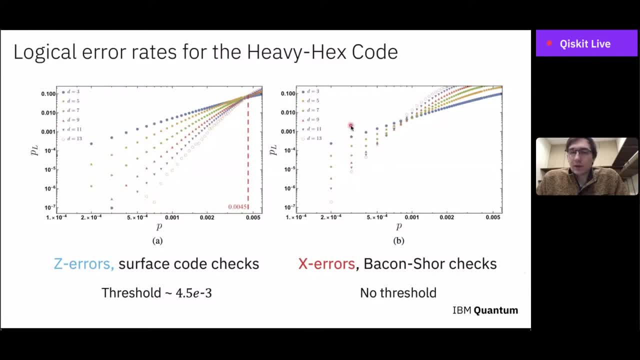 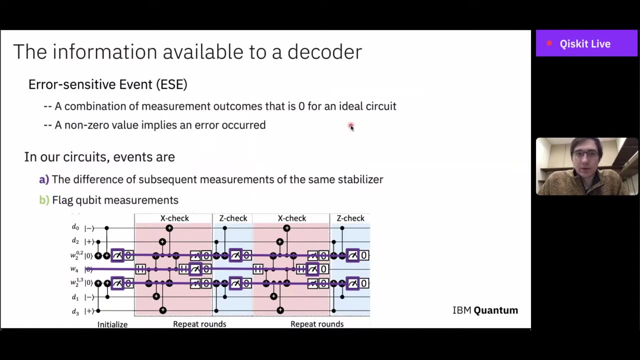 you increase the code size, so it's. so it kind of has this, this pseudo threshold behavior, okay, so i just want to point that out, okay. so now i'm actually i'm moving on to the third part, essentially at the top, um, and this is all about decoding. 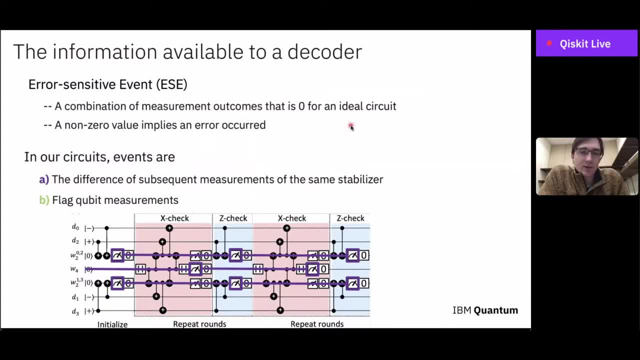 okay, so the the challenge of decoding is taking these measurement results. um, you know, i showed you the measurement circuits earlier. take those measurement results and uh try to figure out what error occurred, right so so. so, in general, the information that's available uh to a decoder is what we call an error sense, a set of error, sensitive events. 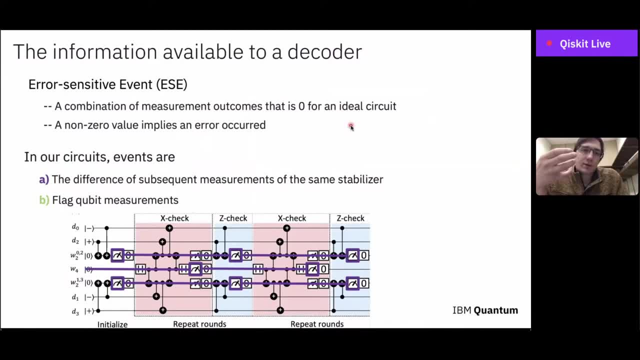 um. so these error sensitive events are some combination of measurement outcomes. that would be a zero if you had an ideal circuit. there were no errors in the circuit, um. so therefore, if you see a non-zero value, then it means that an error occurred. um so so in in the circuits that we do, where we, you know where we initialize some uh logical. 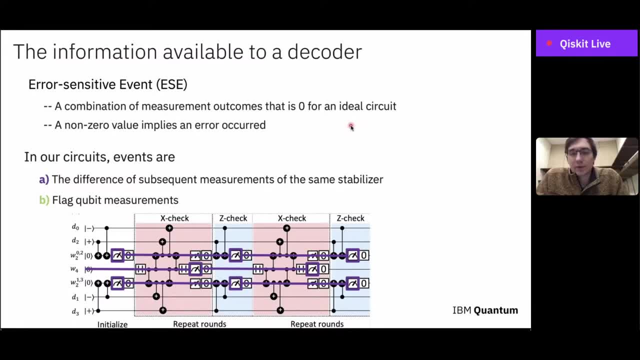 state of the, the error correcting code, and then we repeat rounds of parity check measurements. uh, the error sensitive events are the difference of subsequent measurements of the same stabilizer. so that's what i'm trying to indicate here. um where um right? so so if you look at the z checks, for instance, 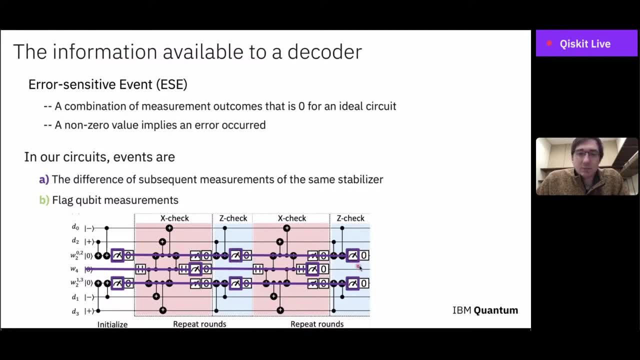 the difference of this z check and this z check would be would make an error, since um, and likewise there's the. there's this first z check where you initialize uh, and the difference of that would be with this z check in the middle as an error sensitivity, um, so the, the x check. 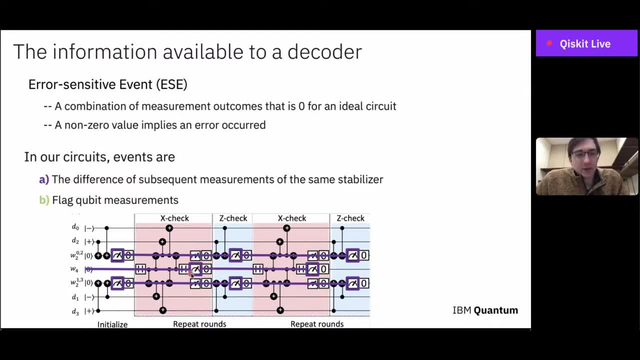 differences as well are error sensitive events. um, and then, in this case, technically, we we have initialized um to an eigens, to it to the well, in this case, the minus one eigenstate, uh, minus one logical eigenstate, but also plus one eigenstate of the x. check um. 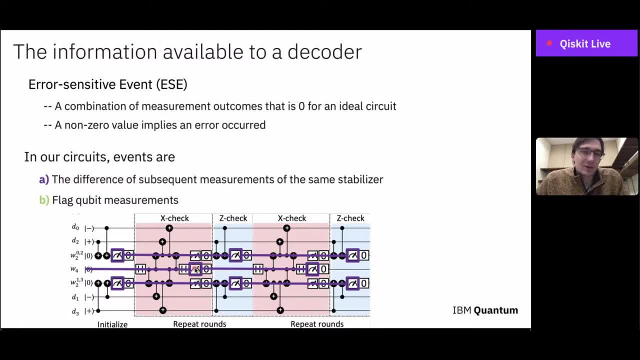 so the. so actually, the first time we measure the x check, we expect to get zero, um, so that that by itself is an error sensitive event. okay, so these are some details, but um, essentially the difference of subsequent, and then the, the. the easier case that we used to draw is that, uh, the flag measurements. 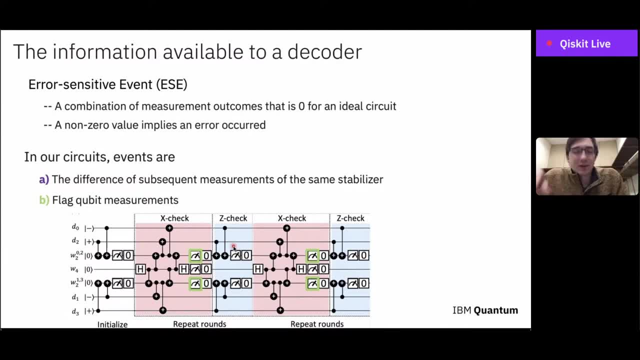 themselves are error sensitive ones. um, so i think you could have picked that up, uh, from from my previous drawings of the circuit. uh, the the flag measurements are always zero if the circuit is ideal. um, so that makes them error sensitive events, okay. so what do we do with these error sensitive events? well, they 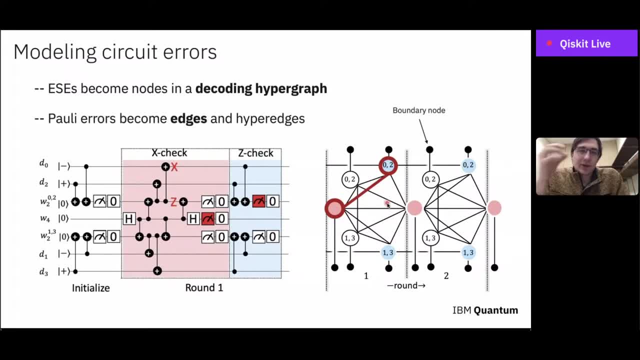 they become, uh, nodes in what we call the decoding hypergraph. so so there are the vertices here, and then, when there are poly errors in the circuit, uh, those become edges and hyper edges in the, uh, in the decoding graph. okay, so let's look at a an example here. um, so these are sort of the 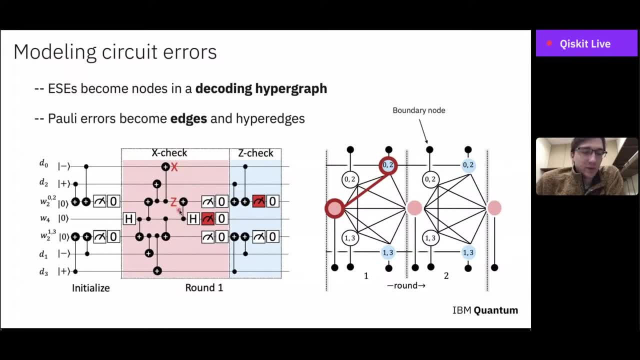 example, cases that we, that we study in quantum fault tolerance. so, uh, that is, we look at poly errors that happen after the different circuit components. um, so here there's a c knot and maybe after the c knot, uh, we experience a z- x error, where there's an x on the target and a z on the control, and then you can propagate this poly. 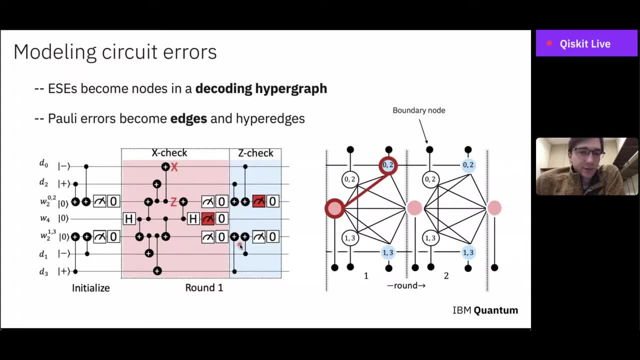 error through the circuit, because the circuit's what's called a clifford circuit. you can propagate it through the circuit and it remains a poly error. and if you do this, uh, you see that this poly error propagates such that it flips these two measurements in red. and when you translate, 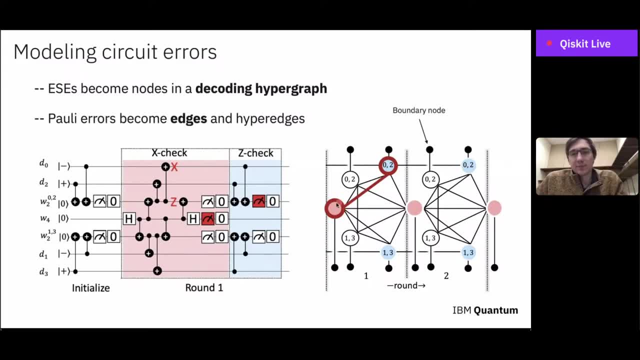 that to the decoding hypergraph. that means that it flips: uh, these two error sensitive events. okay, so because this error could happen, uh, we draw an edge between those two error sensitive events and say that edge represents this error. now, there are other errors that could also draw. 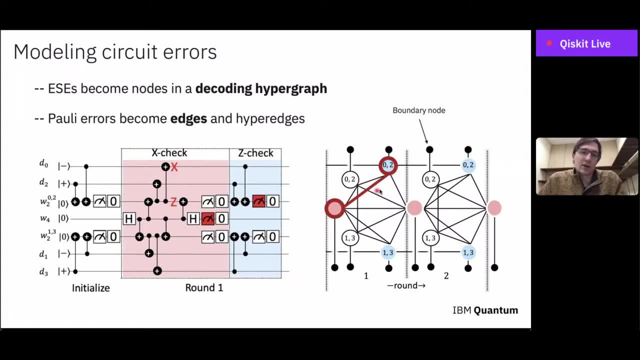 the same edge, um, so so this edge, uh, has contributions from, from different errors actually, um, and then i also want to point out that there, um, there are some errors that trigger just a single node in the graph, and so these get connected to what's called the boundary. 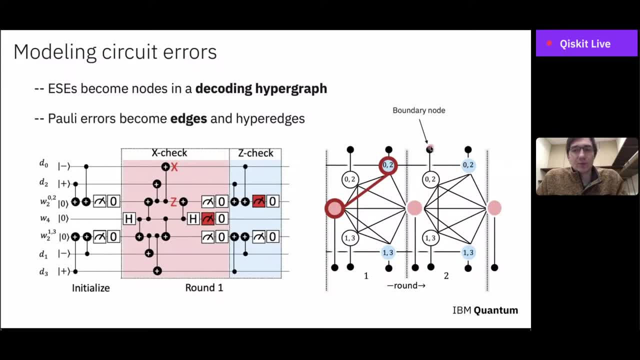 node, uh, just so that we actually have an edge representing, uh, those errors rather than- well, i mean, if it just triggered one event, we can draw an edge. so we introduced this sort of fictitious boundary node so that we can actually draw an edge, and so every boundary node is 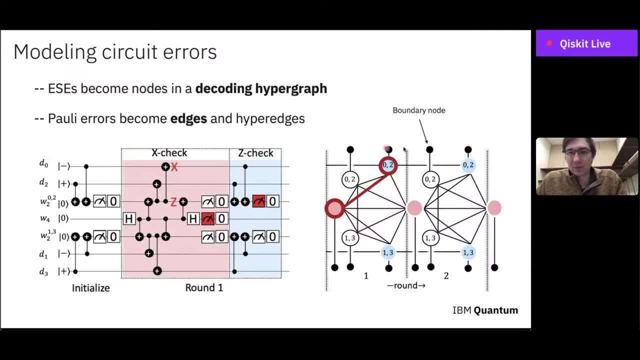 actually the same. do you see that you should think of every boundary node as connected to every other one with, uh, with an edge of weight zero? or you can just think of them as, all the same, some giant boundary node on the outside. okay, so? so that's edges in the decoding hypergraph. 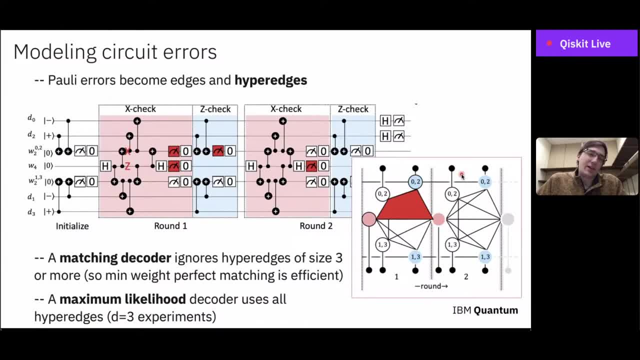 um, but actually sometimes errors occur and, uh, you, you end up triggering more than two error sensitive events. so here's an example: if there's a zx error after this c naught, then it propagates the circuit and it triggers four different- uh, four different- measurements here, and that translates to four different error sensitive events. um, so then we draw a hyper edge. 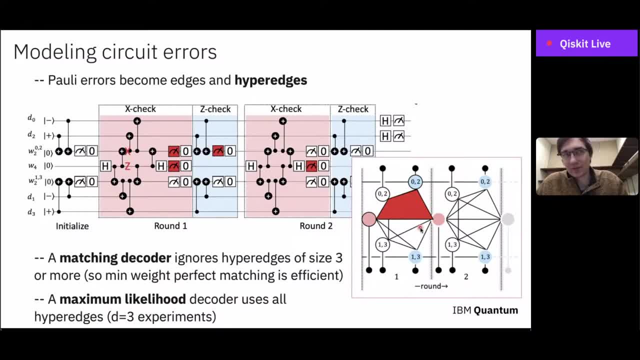 in the decoding hypergraph. well, this is why it's a hypergraph instead of instead of a graph, um. so these hyper edges are are interesting, um, because they're actually- i mean, they're actually real, um. but then there are, there are two different decoding strategies, uh, the first of which, the matching decoder, actually ignores the hyper edges. 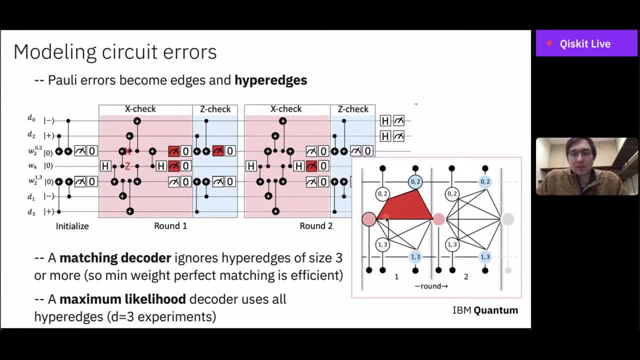 um, so, so if you have a, uh, well, a hyper edge of size three, a hyper edge of size two is just an edge, uh, a hyper edge of size three or more, uh, the, the matching decoder uh ignores this, and the reason it ignores it is so that we can make the algorithm efficient. 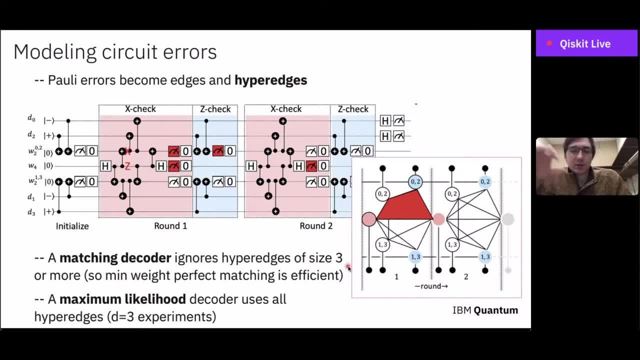 so it's a minimum weight. perfect matching is a problem on these, these graphs where you try to match up, match up a set of highlighted nodes in pairs and you try to do that using the minimum weight paths, and it's efficient. if, um, if you're uh. 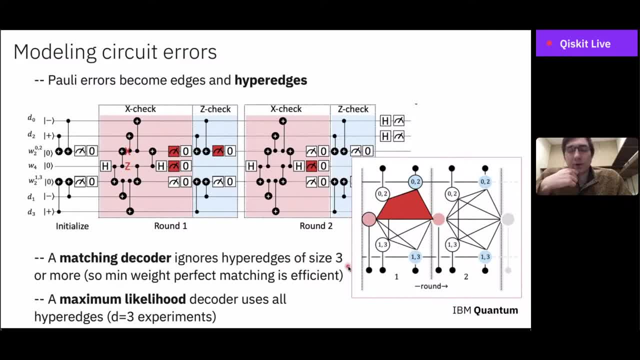 okay, if you're just working with a series of pushes, then you can just replace it along the X boundaries. the advantage of 그게 graph rather than the hyper graph. so this is in contrast to maximum likelihood decoding, which uses all the hyper edges. so that's something that we do in our g equals 3. 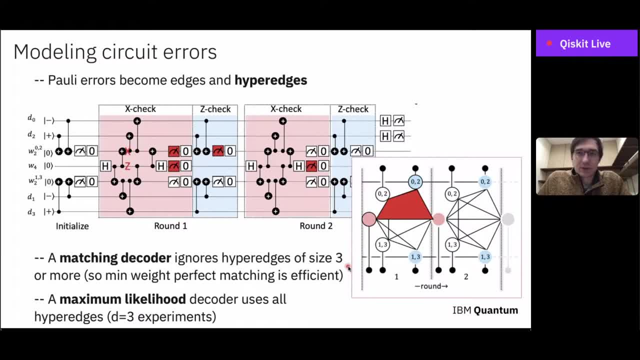 experiments, which I'll explain later. so actually this is. I've been using hyper graphs and graph for this object, so it shouldn't be surprising that this is the most important. graph. number 3: ok, a lot of important graphs, ok. so now I'm going to go through our 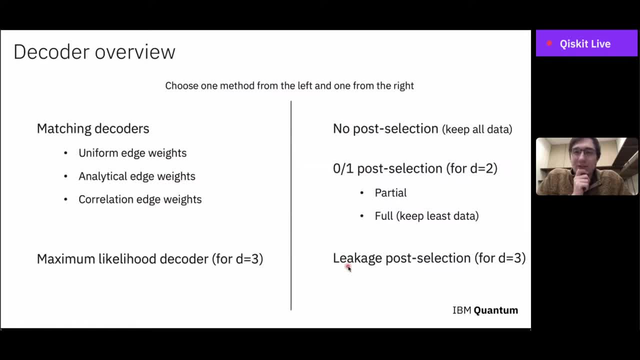 decoding methods for our d equals 2 and d equals 3, experiments actually on IBM. so essentially, this is the overview. you get to choose. you get to choose your algorithm from the left column and you get to choose some sort of post selection method from the right column. 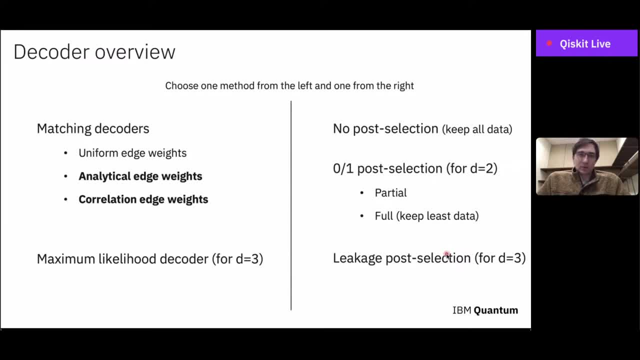 and these are what we look at. so we have the matching decoders before I. so we have the matching decoders, which I explained a bit about, and then we have the maximum likelihood decoding. the post selection strategies range from no post selection, where you just keep everything and try to do your best. 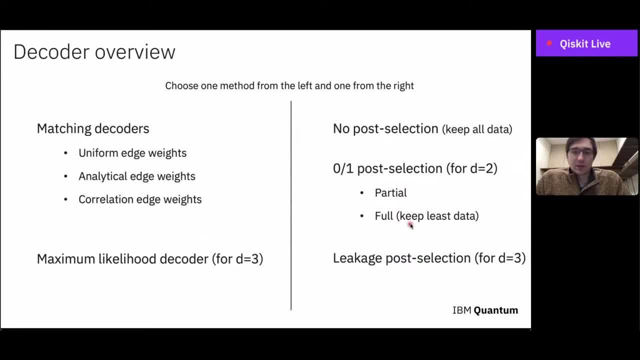 decoding it to something called full post selection, where you essentially throw out every case where you detected any error. so the first thing I'm going to explain here is how we do this matching ok. so essentially the problem, I'm jumping ahead. so this matching decoding, I explained. 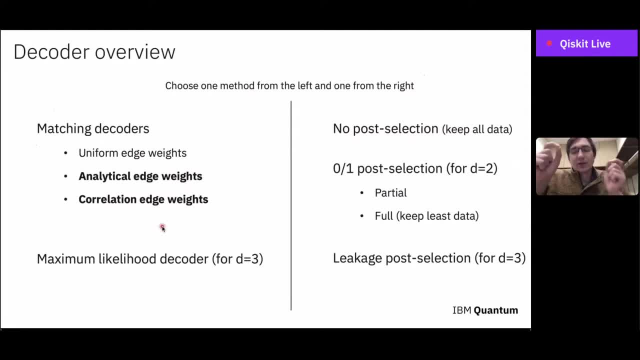 that you you match up highlighted nodes along as a minimum weight. so, essentially, the problem is to set the edge weights to what should be. yeah, I mean, how should the edges be weighted so so that minimum weight, minimum weight quantity is meaningful? so what you could do is set every edge. 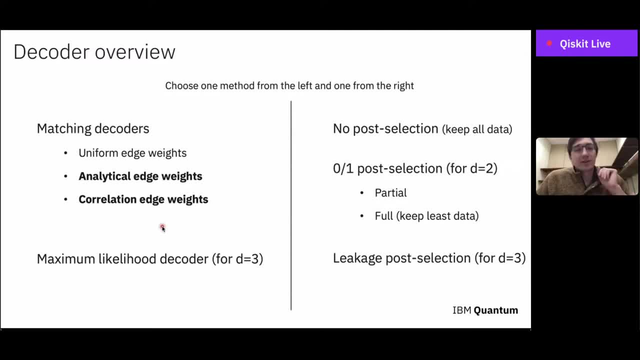 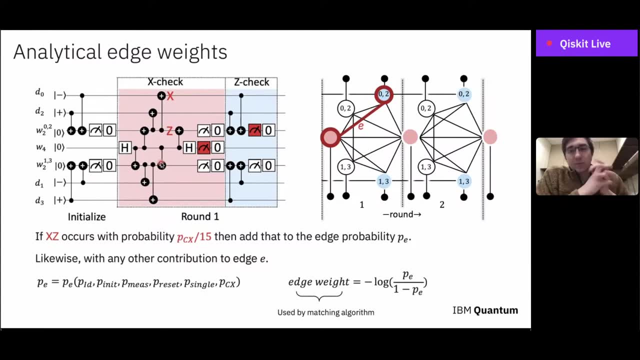 to the same weight. every edge gets weight one. that's the uniform edge weight method, so I'm not going to explain more about that. But the analytical edge weight and correlation weight methods are a bit more complicated. So what you do in the analytical weight method is that you look 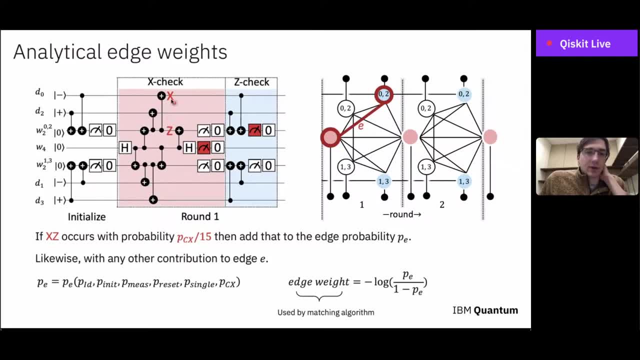 at this error, as we, you know, as we, as I showed earlier, if this xz error occurs with some probability, then you add that probability to the probability of an edge. okay, So the probability of an edge is related to the weight of the edge as follows: So the edge weight is equal to minus log. 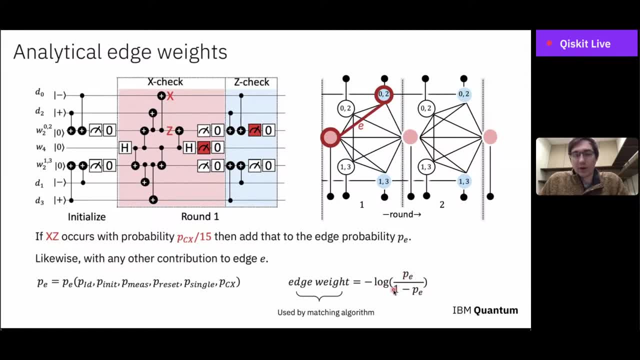 of the probability of the edge over one minus probability of the edge, And essentially why it's this is that now, when you add the edge weights up, you're multiplying the probabilities. Okay, so then the total edge weight ends up being the like log probability of that of those edges. 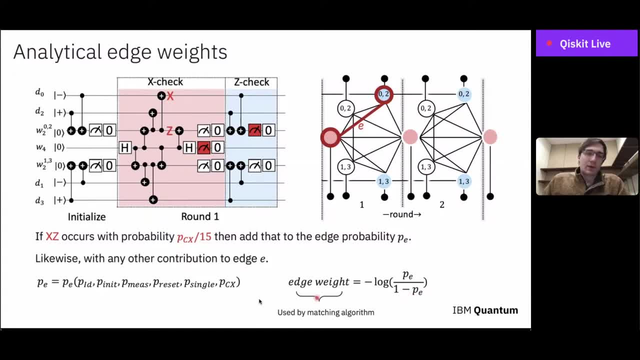 And so the edge probability ends up being a function of the probabilities of various circuit components failing, And we assume that these are just fixed numbers for every component, like every CNOT in the circuit, fails with probability PCX. This is like the theorist model of this. 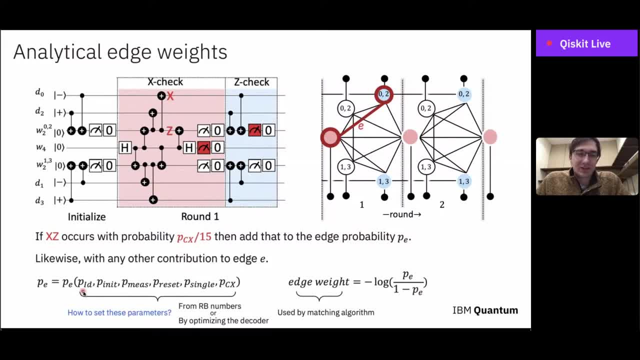 So then the question becomes: how do we set these parameters, the probabilities of various circuit components failing? And you could do this from randomized benchmarking the components, or you could do this by optimizing the decoding, So you tune each of these parameters until the decoder does as well as it can. 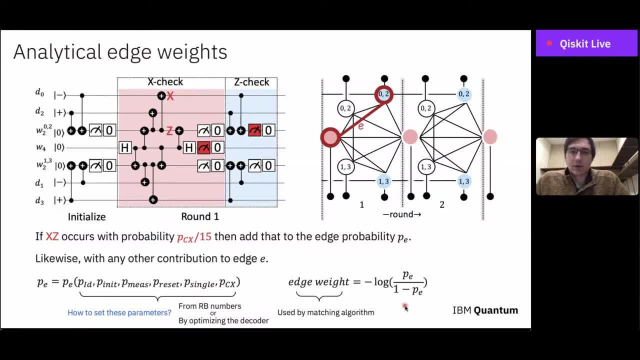 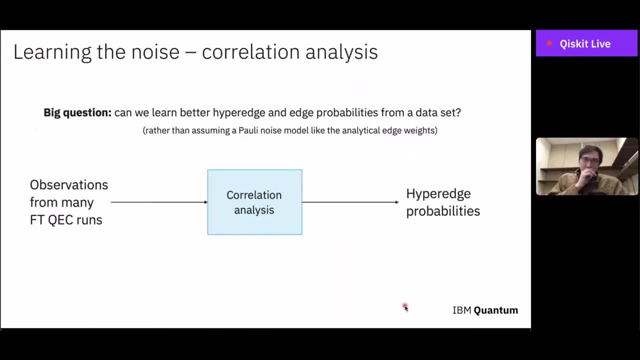 So those are two strategies to set edge weights in the analytical path. Okay, so now That was the analytical method, which is like, in theory, how we expect errors to work right. So then, the big question is: could we learn better edge weights by looking at our actual experimental data? 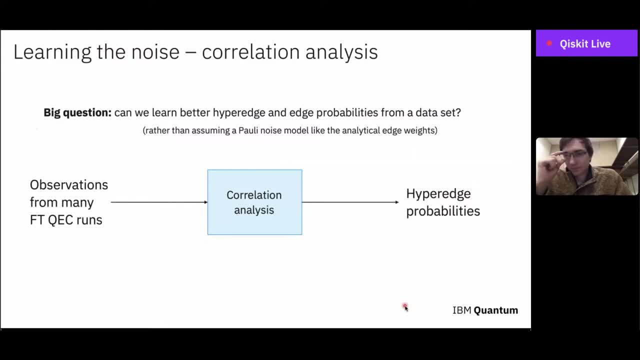 So that's what this correlation analysis tries to do, It's like. rather than assuming the poly noise model from the previous slide, let's look at the real data. So here's a schematic of what's going on. right, You take observations from many of your runs of the experiment, where you're doing these repeated parity checks, and plug it into the correlation analysis. 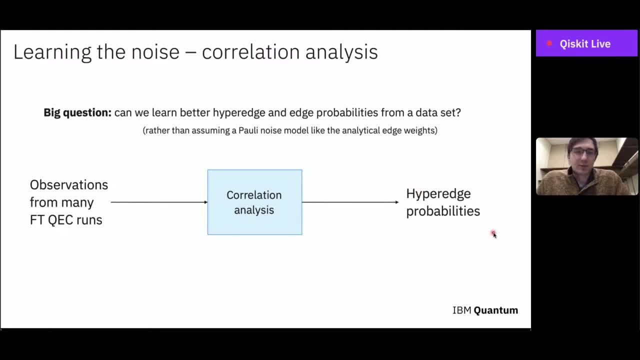 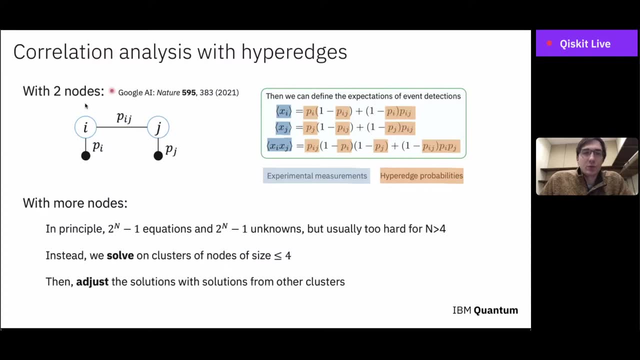 And then, hopefully, you get out some hyper-edge probabilities that make sense So roughly. how does it work? Well, here's a two, two-node example, which you can find from this Google paper. So there are just two nodes, but that means that there are three edges. 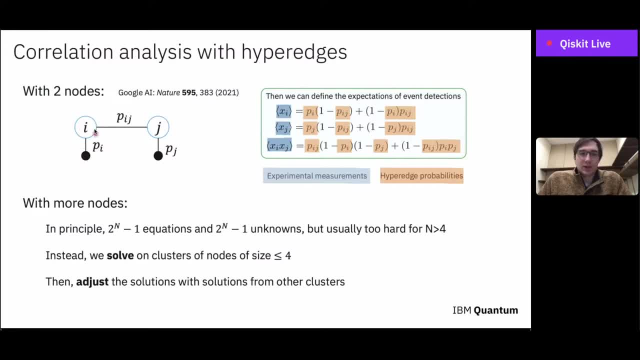 There's the edge from node i to the boundary, There's the edge between i and j And there's the edge from node j to the boundary, And you can write the expectation values, so the expectation that this node is triggered or this node is triggered, or both, in terms of the probabilities of each of these edges. 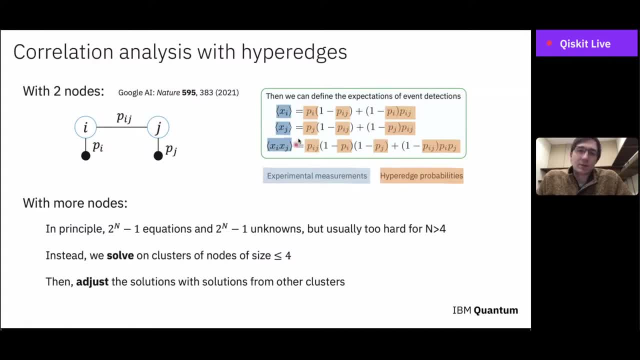 So that's these equations here, And so what you get from the experiment is some expectation value Or these expectation values on the left, and then you can solve for the probabilities on the right, And so just invert these equations. Now, if you generalize this, 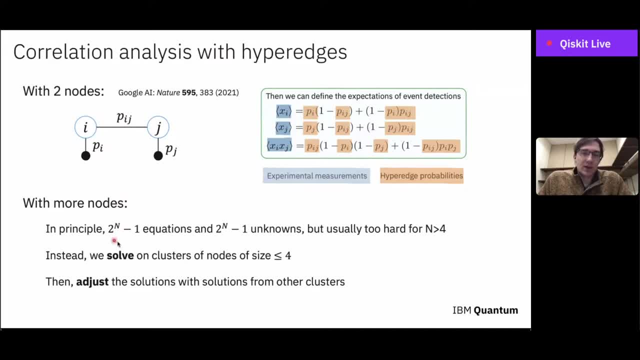 you're going to end up with two to the n minus one equations if there are n nodes, And you're going to end up with two to the n minus one unnodes, So you can try to solve these equations numerically rather than inverting it exactly. 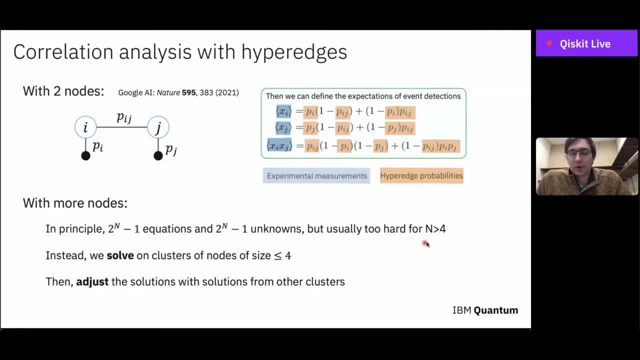 But this even becomes too hard for n-graded people. So instead what we do is we solve these equations. These equations on what are called clusters of nodes, where we just assume that nodes in the cluster exist, So clusters of size four. We just assume that these four nodes exist. 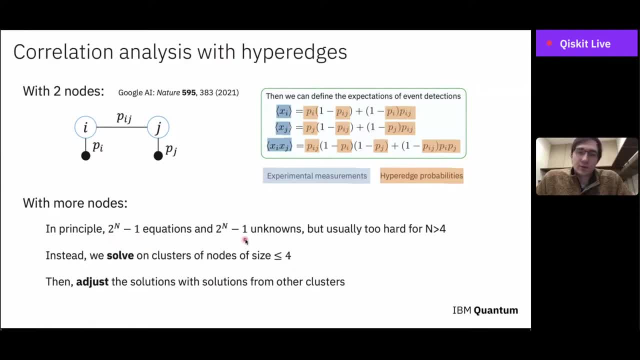 And we just end up with 15 equations, 15 unknowns. Solve that And then you can adjust the solutions you get from that with solutions from neighboring clusters. Okay, so that's roughly how it works And I'm not going to explain more. but you can click on the papers if you want. 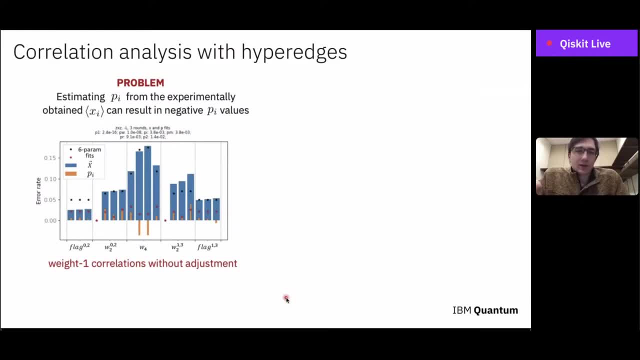 So just to indicate that this actually is doing something meaningful, here is the case where we're estimating the edge probabilities for the nodes connected to the boundary. So here are all the edges Where one side of the edge is the boundary, And if you do this without taking into account the larger size hyperedges, 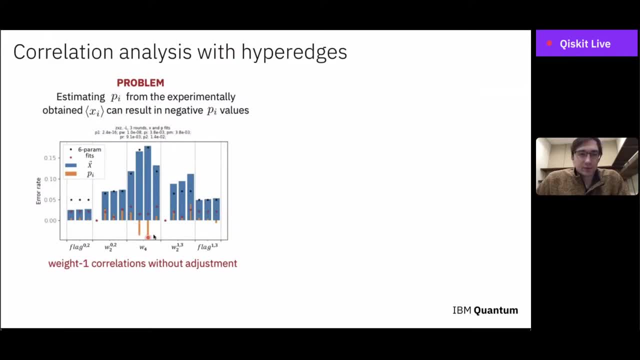 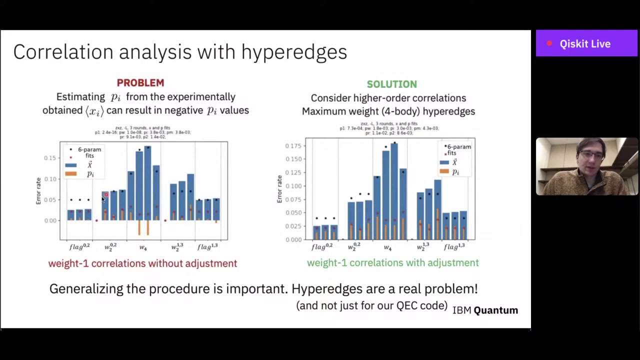 then you end up with negative probabilities here. So I think p sub i is the probability you get out of the correlation analysis, And then the other value is the expectation value of p, The expectation value of x, And then there are some analytical values which are the points. 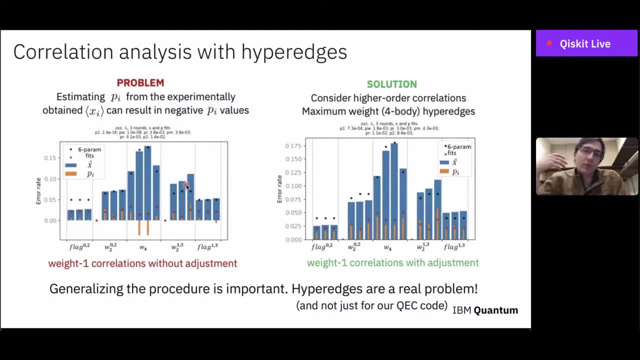 Right. but if you do take into account the larger size hyperedges, then you can get rid of these negative estimated probabilities And from the same data set you get better estimates for the the edge probabilities. Okay, so this indicates that generalizing procedure is important. 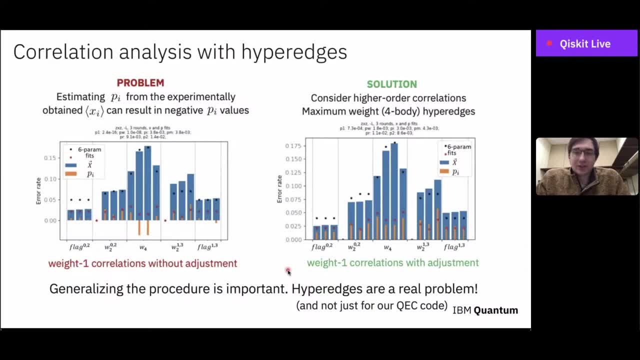 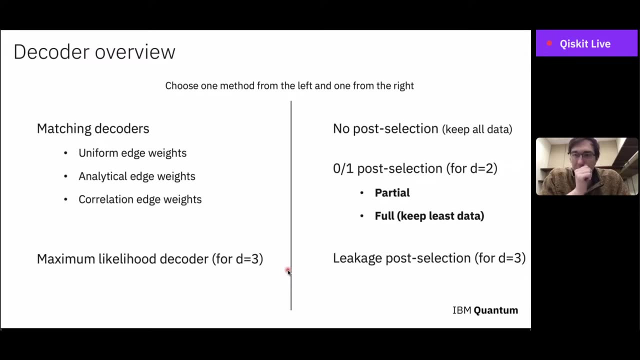 The hyperedges are actually real, And this can occur in other quantum error correcting codes too, So I think this is important. Okay, so that was the analytical and correlation methods. Now I'm going to explain how we do some of the post-selection. 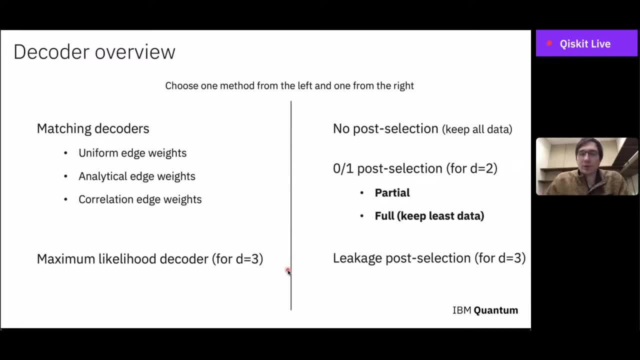 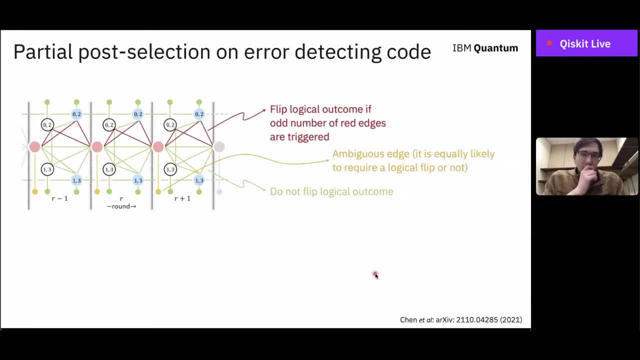 strategies. So obviously the no post-selection is straightforward. Let's just jump to this category 0, 1 post-selection, which is just to differentiate it from the leakage post-selection. Okay, so essentially I need to explain another property of the decoding graph. 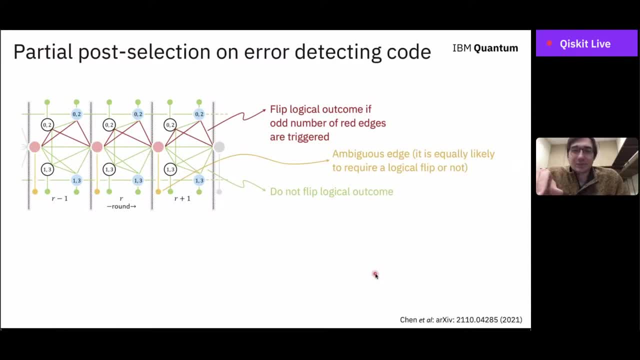 which is that every edge is also colored. So if it's clear, if it's colored red, that indicates that if the matching algorithm chooses that edge, then you have to flip the logical outcome, And if it's colored green, then that indicates that you don't flip the outcome. 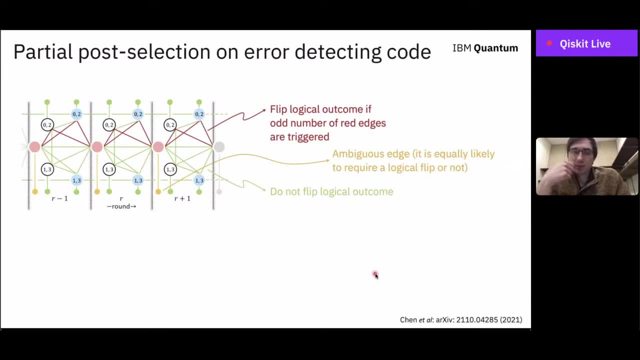 And if it's colored yellow then it's ambiguous, So it ends up being 50-50, whether you should flip or not flip, And the existence of these ambiguous edges is just because we're looking at the D equals 2 code here. 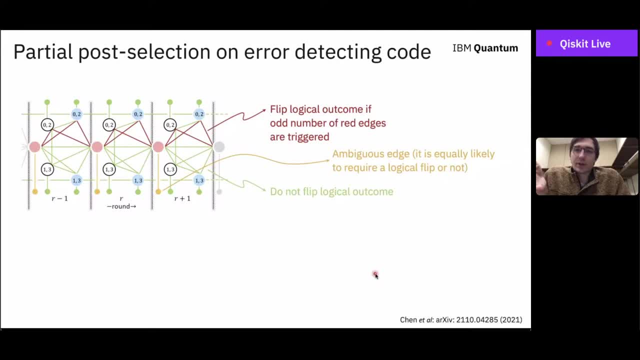 what's called an error-detecting code, because it detects one error, but it can't necessarily correct every single error. So some edges are ambiguous, And so this gives rise to our two post-selection schemes here. So if you do full post-selection- 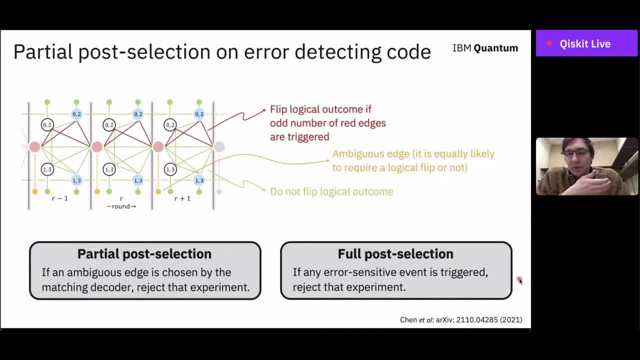 what that means is that if any error-sensitive events is triggered, then you reject the experiment. So this is the most brutal right. So this is going to cut out as many experiments as you can, And it also leaves you with sort of nothing interesting going on. 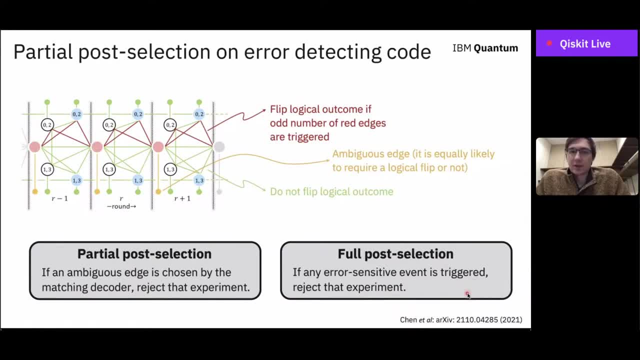 So any experiments you keep just have zero measurement. You measure zero for all your RHI. So that means we can't really study decoding algorithms if we're doing full post-selection. In contrast, if we do partial post-selection, where we only throw out an experiment, 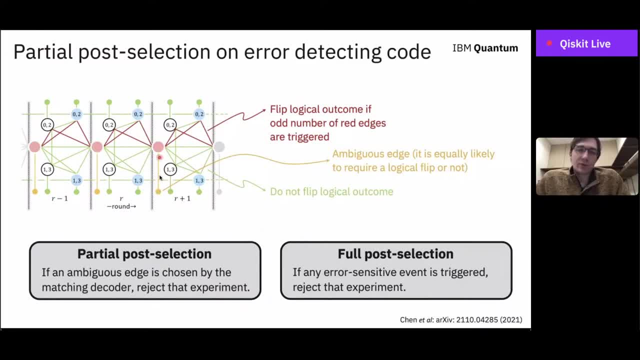 if the matching decoder chooses an ambiguous edge, because otherwise we know how to correct- or at least we do- if there was just a single error. So we only need to throw out cases where it chooses an ambiguous edge. so the decoder is allowed to say that it's uncertain. 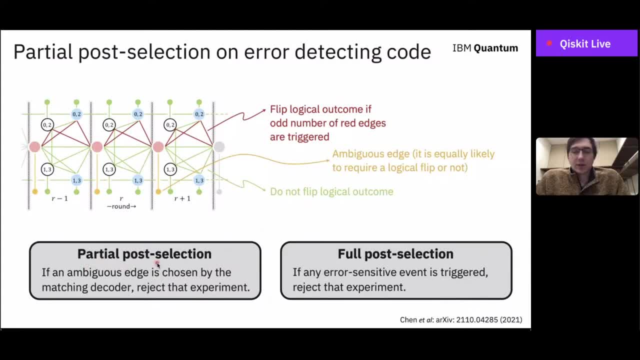 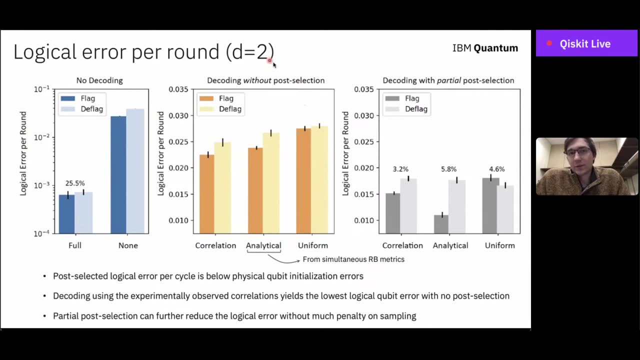 So if we do this partial post-selection strategy, then we're actually keeping interesting cases and we can look at our decoding algorithms and compare them. So that's what this slide is communicating. our final results for the D equals 2 code. on the left, there's no decoding. 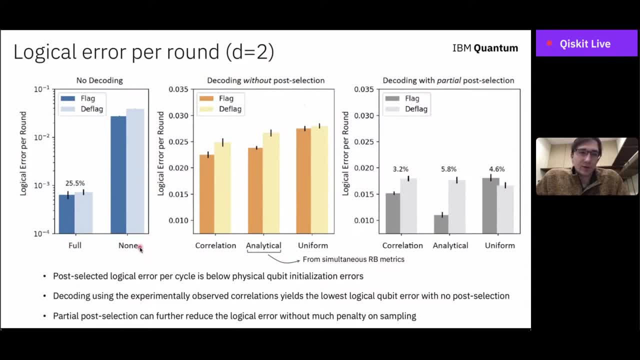 and there's either full post-selection or no post-selection. The percentage here is how many experiments are thrown out due to the post-selection. So here we throw out like 25% of the experiments if we do full post-selection And then also whether we do this deflagging procedure. 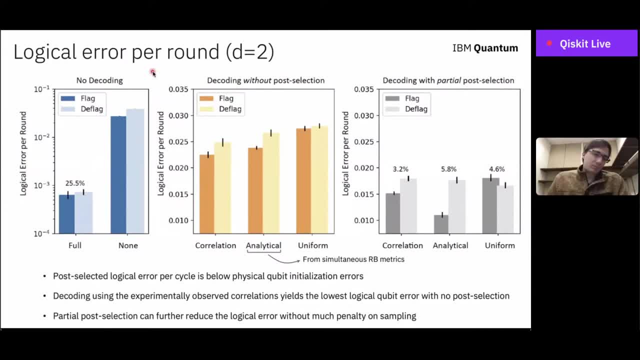 that I talked about earlier, or not, Right? So in the full post-selection case, we get error rates for the logical qubit that are below, like 10 to the minus 3, which is even exceeding our physical error rates If we don't do any post-selection. 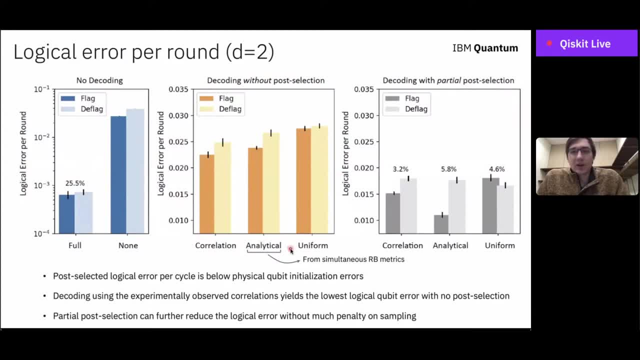 so this is keeping all the results, and if we match along an ambiguous edge, then we just say that we don't flip the logical. then we see that the correlation decoder is outperforming the analytical by a bit. And if we look at decoding with partial post-selection, 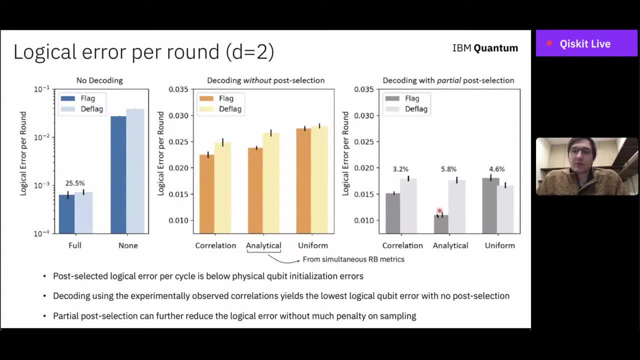 then the analytical is actually performing the best. So these are our results for the D equals 2 experiment, And now I'm going to move on to the D equals 3 quickly. We have about five minutes left. Here's the D equals 3 circuit. 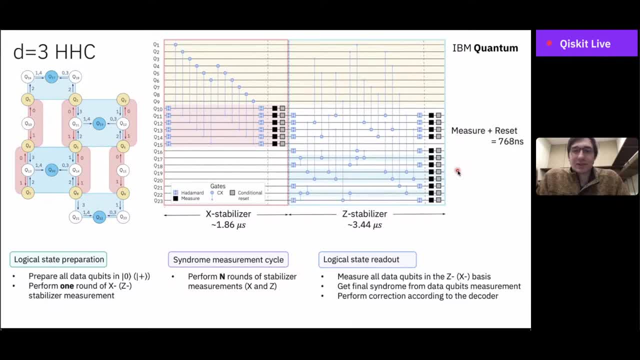 It's just a bunch of concepts. It's a bunch of copies of the D equals 2 circuit, So I'm not going to spend too much time here. But essentially, again we have a logical state preparation And then we have repeated rounds of parity check measurements. 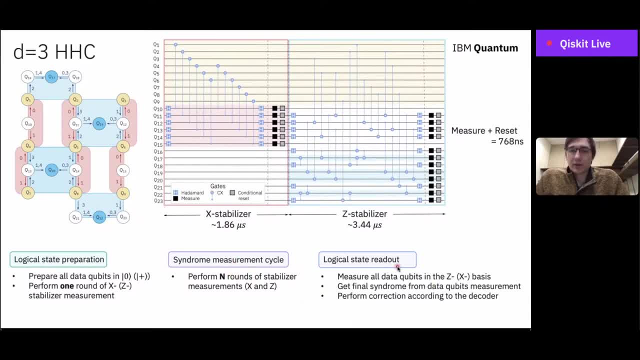 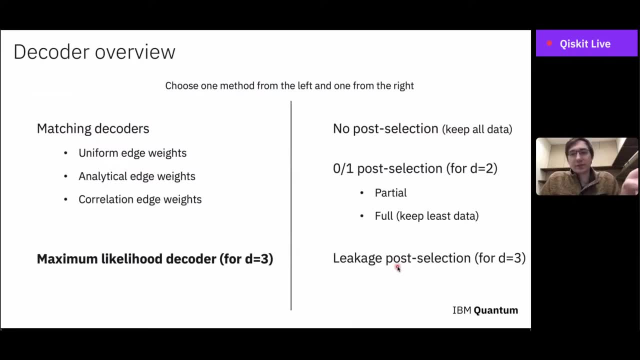 or syndrome measurements, And then finally, we end with a logical readout of the state. So what's unique for our D equals 3 experiments is that we tried out this maximum likelihood decoder. Well, also, we tried out the leakage by selection. 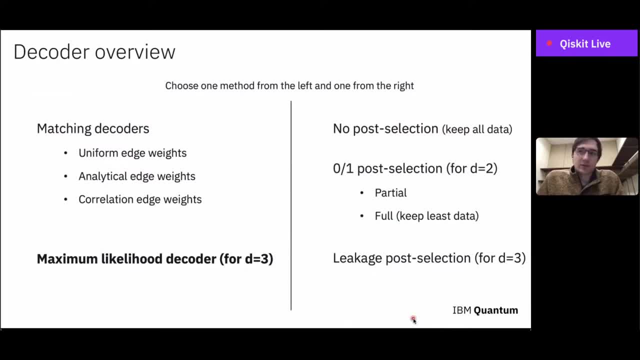 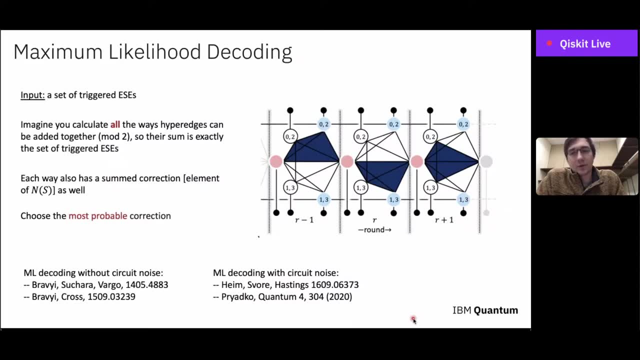 So we have to discuss both of these before getting to the results. So here's the maximum likelihood decoder, or at least an overview of it. I'm not going to go into more detail than this, actually. So the input is the set of error sensor events that you see. 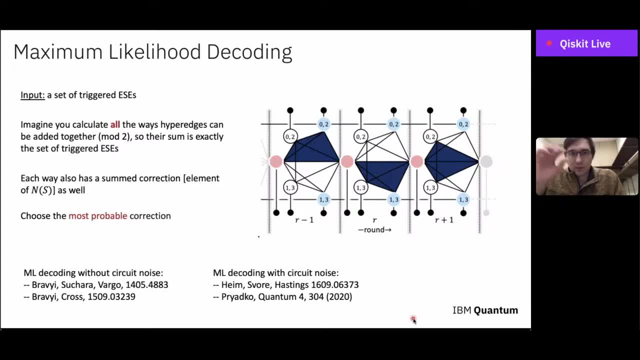 But then you imagine that instead of just doing this perfect matching that the matching decoder does, you actually imagine that you take all the different ways the hyperedges can occur, so that when you add together that subset of hyperedges their sum is exactly the set of error sensor: sensible events. 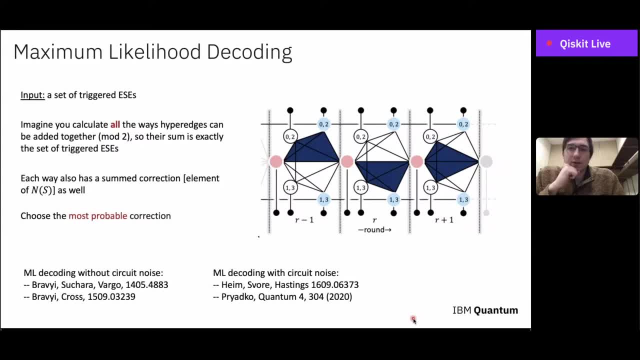 that you see. So you look at all these combinations that give you the observation that you see, And then each of those combinations also tells you some correction to apply, And then you just choose the most likely correction. So this is an exact maximum likelihood decoder. 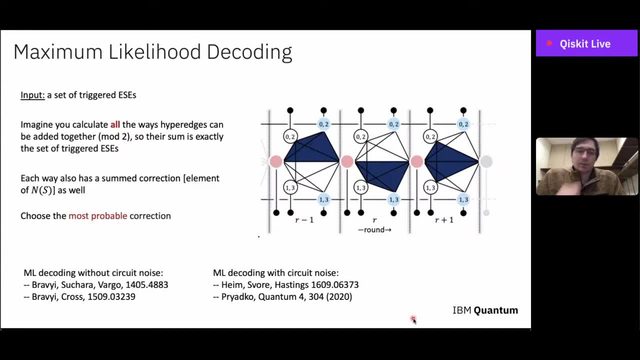 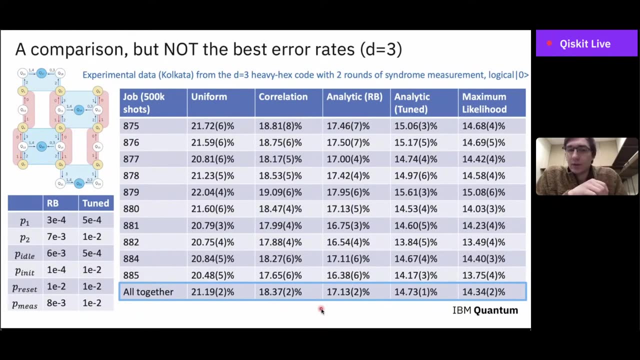 for circuit noise, which is kind of in the spirit of these two papers, Lyme Soiree and Hastings, and also Preacta. So again, the maximum likelihood decoder is taking into account the hyperedges, whereas the matching decoder is not. 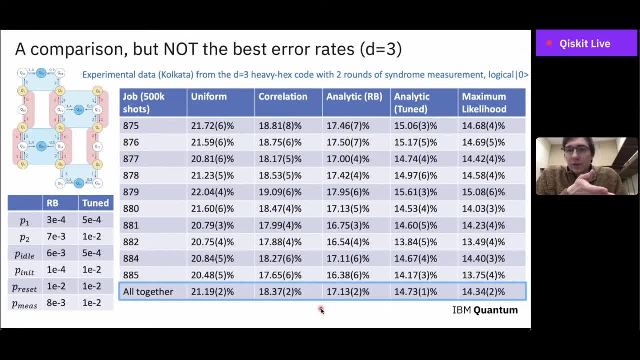 So we expect improvement. So that's what we see in this experiment on our Cortada device. This was sort of a preliminary experiment where we compared all the different decoding methods for our G equals 3 code And we see that the maximum likelihood decoder 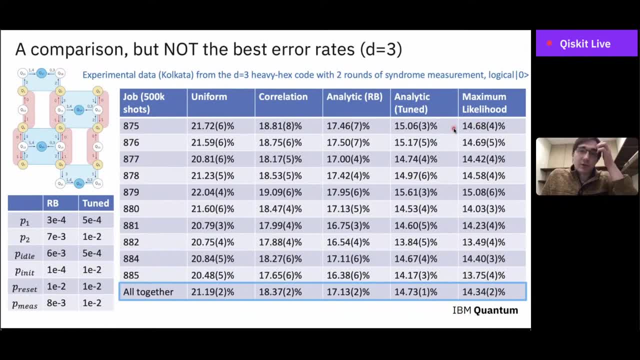 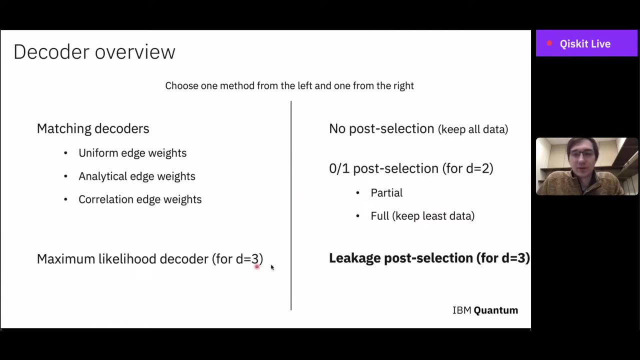 is performing the best, And followed closely by the analytic model where we tune the parameters of the noise And so we tune the parameters so that we're getting the best decoding possible. So that was the maximum likelihood decoding, which we'll return to for our final results. 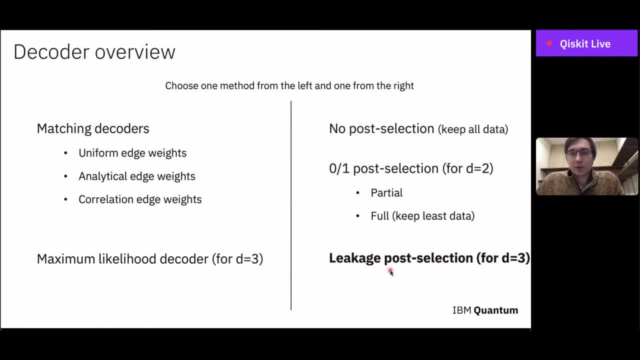 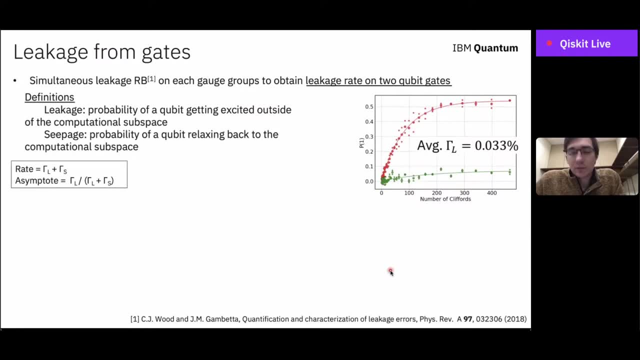 But now I want to discuss the leakage post-selection. So what is leakage? So I mean in our qubits there are actually more energy levels than 0 and 1.. 0 and 1 is used for the qubit, But then the state could also leak to levels 2 or higher. 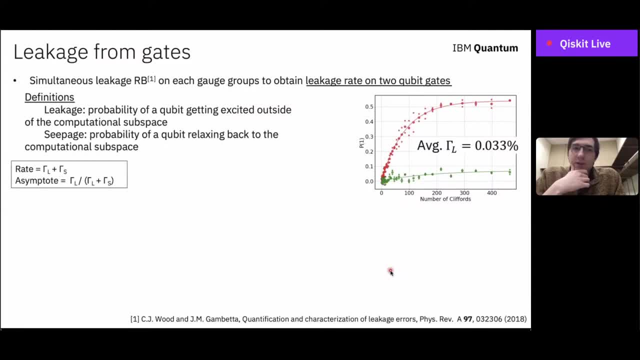 So that's leakage out of the computational space. So there are certain ways to characterize leakage, So you can characterize leakage in the device, And essentially these amount to repeating the circuit element many times that you want to characterize. So you can repeat the gate many times. 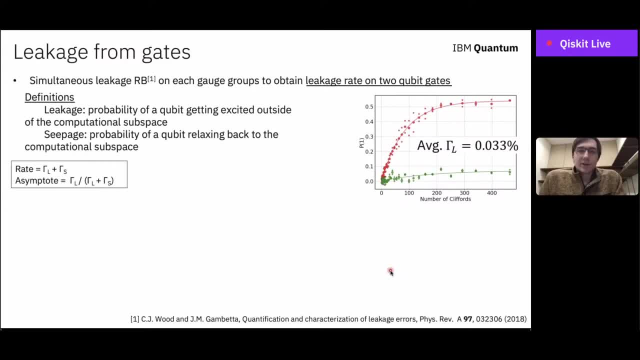 and see how often it leaks right Or see the rate of leakage. So you get sort of plots like this where as you repeat the gate, the amount of leakage goes up And you can fit to this curve, this P-leak. 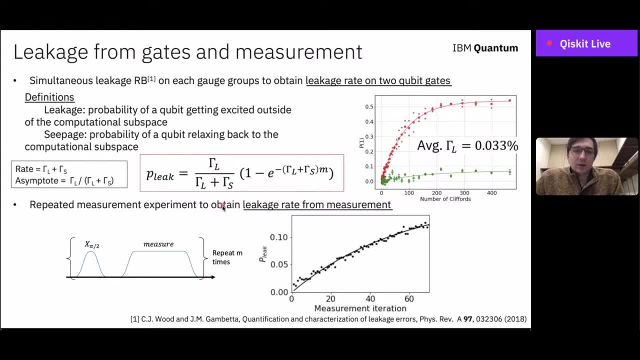 And from that you get the leakage rate, gamma sub L. You also get what's called the seepage rate, which is the probability of the qubit goes back into the computational space. So you can do this for both gates and also for measurements. 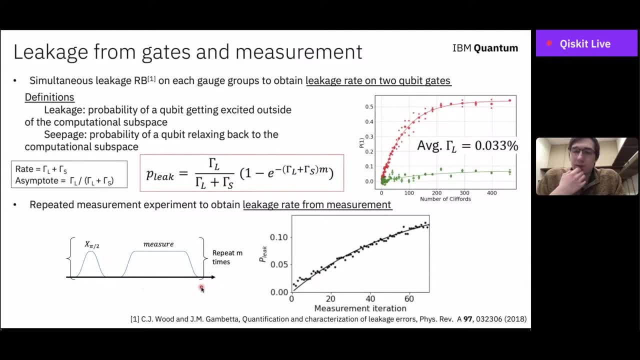 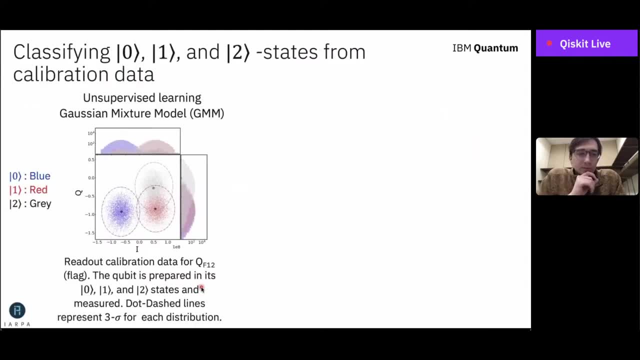 The measurements you repeat multiple times, just as you do for the gate. So this way you can estimate your leakage rates. Now, this should not. yeah, okay anyway. So this: when we do our experiments, what we want to do is actually characterize a single measurement. 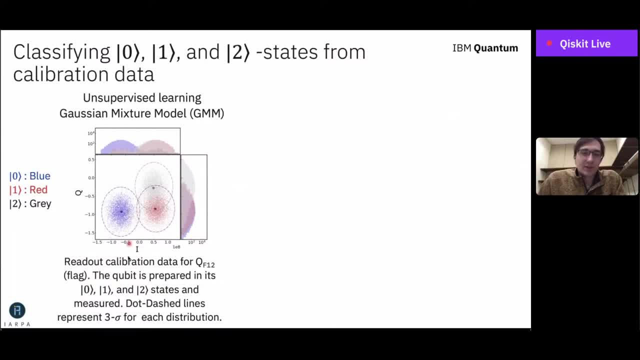 So the single qubit measurement gives us some point in this IQ plane, which we can characterize as either 0,, 1, or 2.. So, for instance, we get some plot that looks like this And the qubit is prepared. 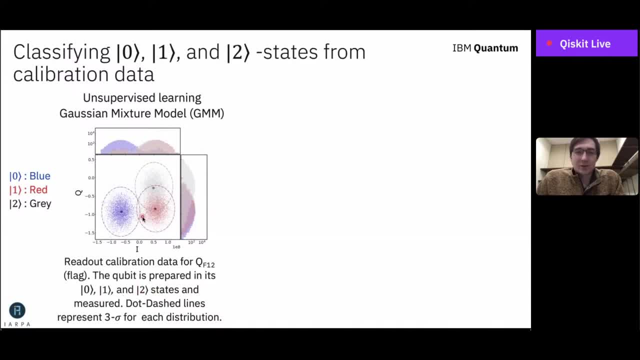 So the way you generate this plot is by preparing the qubit in 0,, 1, or 2, and then measuring it repeatedly, And so there's some mean and standard deviation of the I and Q values that you get for each of these preparations. 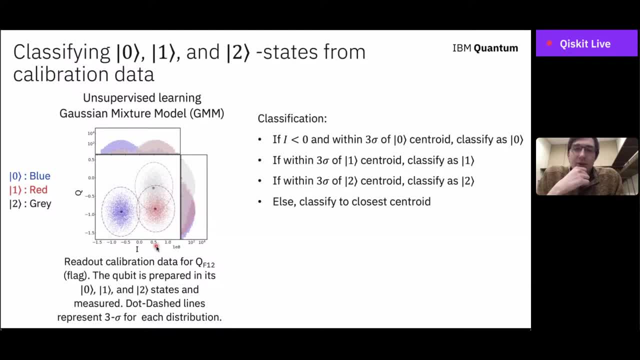 And so the way we propose to classify a certain measurement is that if I is less than 0, and you're within 3 sigma of the 0 state, so in blue here- then you would classify the measurement as 0. And then, if that's not true, you check the second condition. 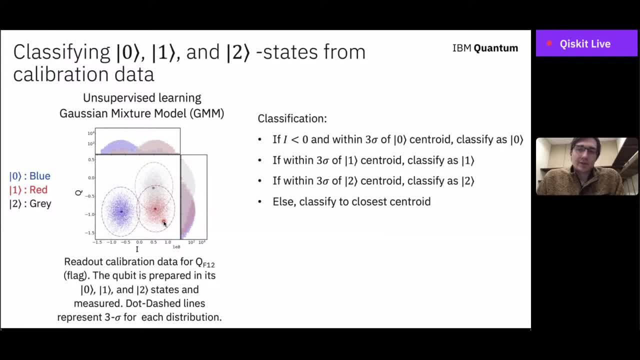 If you're within 3 sigma of the 1, classify as 1.. And then you check the third. If you're within 3 sigma of 2, classify as 2.. Otherwise you classify to the closest. So why do you want to do this multi-step procedure instead of a single step? 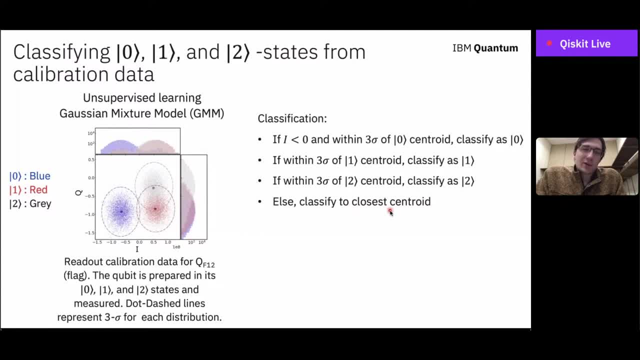 So like a single step could just be. let's say, we want to classify to the closest centroid, right off the bat. Well, we do this multi-step because here we're prioritizing the one states which you know, because we start the qubit in the computational space. 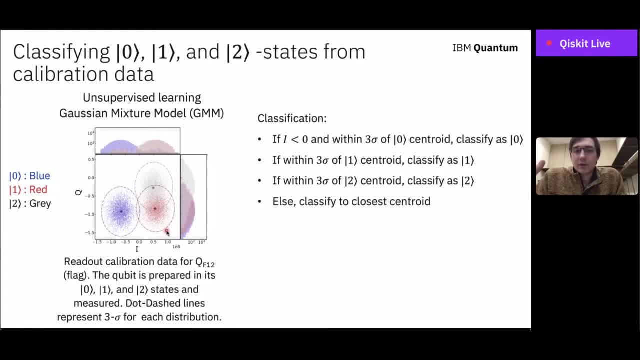 we sort of expect. there's some prior belief that we are going to remain in the computational space most of the time And there's great overlap here between the one and the two. So we want to make sure that we're classifying the one more often than we're classifying to the two. 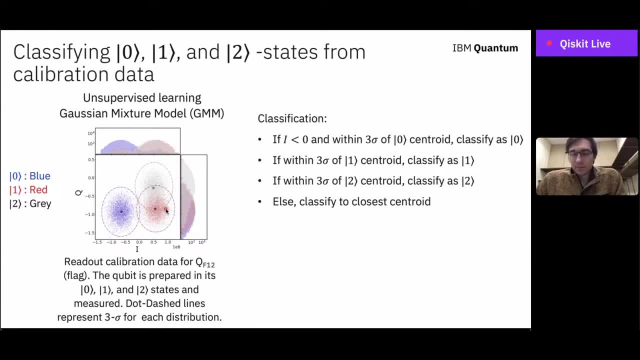 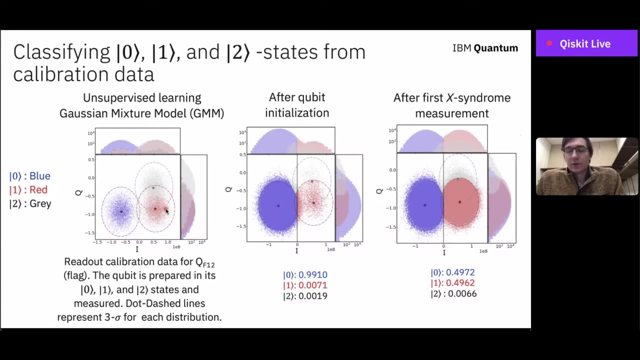 because that's just more likely based on our prior belief. Okay, So here's some examples of you know, if you initialize the qubit, it gets classified to zero state, most often After you do a cinder measurement, where it's 50-50,. 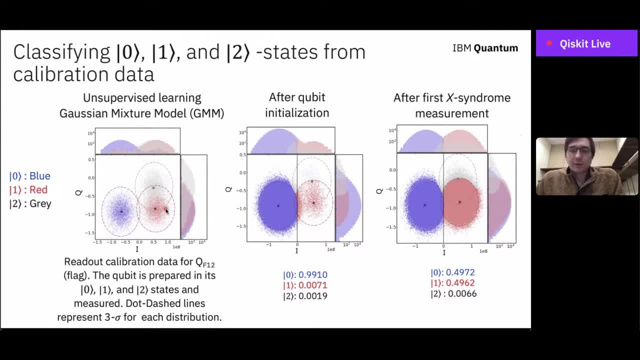 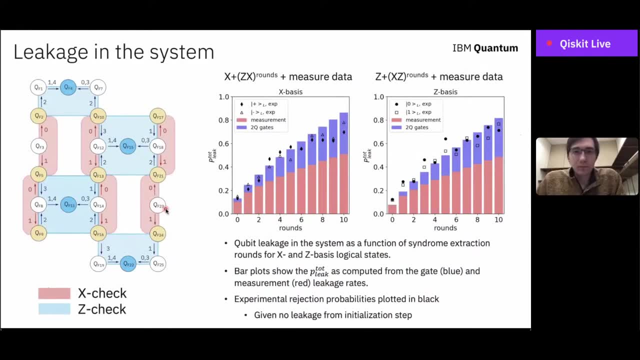 whether it's 0 or 1, it's roughly 50-50,, 0 or 1.. Okay, So this slide is just communicating that when we do this classification method for our rounds of parity check measurement, this leakage classification method. 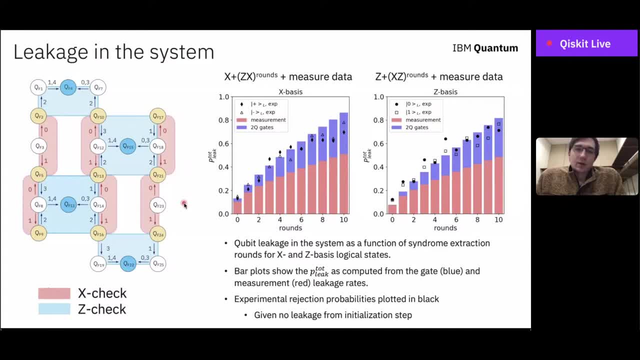 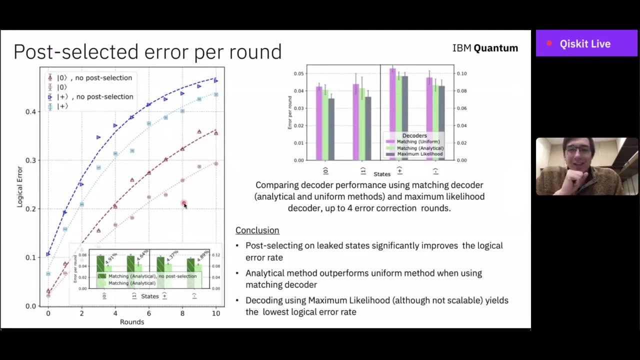 we're getting values that are roughly the same as what we expect from our leakage characterization. Okay, So these are roughly matching up, And this is like the second to last slide, so I know I'm a bit over time. So here are, like some of our final plots. 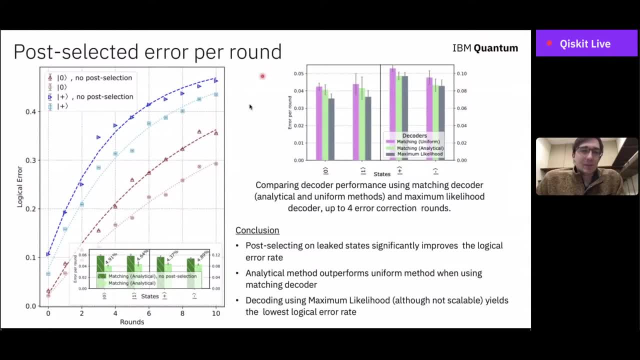 for the D equals 3 experiment. Here we have the logical error rate as a function of rounds And essentially by fitting these curves you can get the logical error rate per round which is shown in the inset here, If you do post-selection. 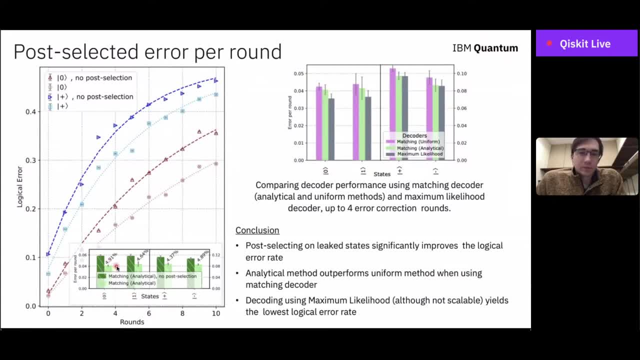 where we throw out, you know, 4.3 to like 5% of the data. then you actually get improved logical error rates by 2% or 4% in the case where you're starting in logical plus or minus. Okay, 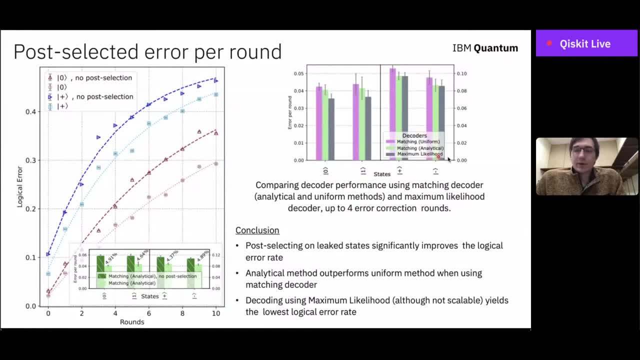 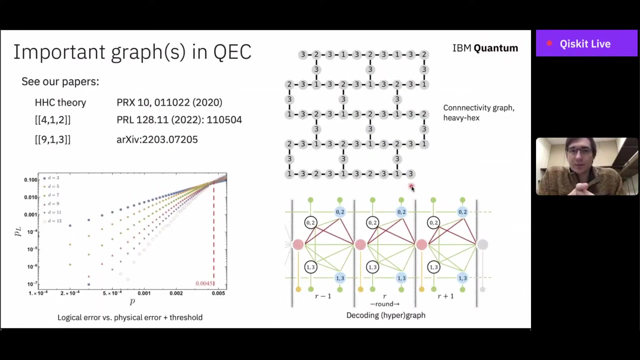 And then we can also compare the decoding strategies. So here we have a couple versions of the matching decoder and then the maximum likelihood decoder, And the maximum likelihood decoder is improving over the matching decoders. Okay, So I want to conclude here, because I'm over time. 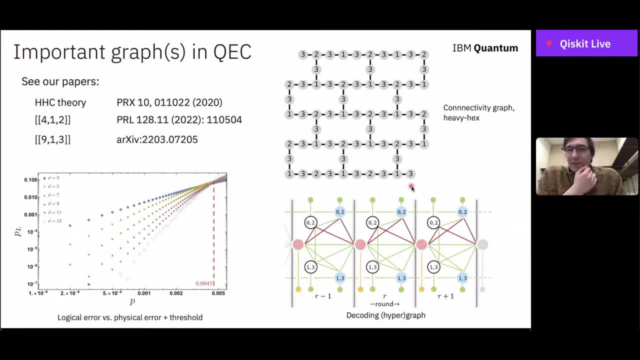 but this is my summary slide of the most important graphs in quantum error correction. You can see the logical error rate plot, the connectivity graph and then also the decoder And then also the decoding graph And you can check out our papers. So thanks for listening. 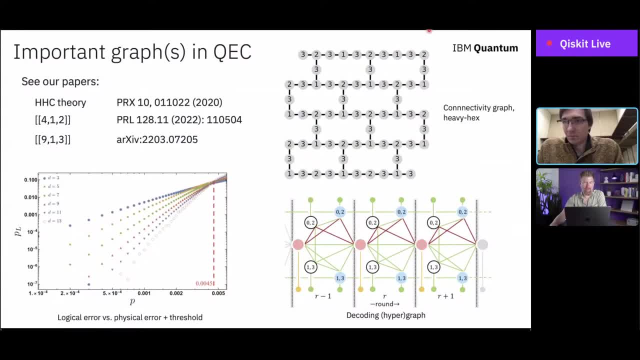 and I'll happily take any other questions. Well, thank you so much, Ted, for that wonderful talk. That's definitely a fascinating topic and you've touched on so many aspects of quantum computing. Could I get some applause emojis in the chat and any questions you might have? 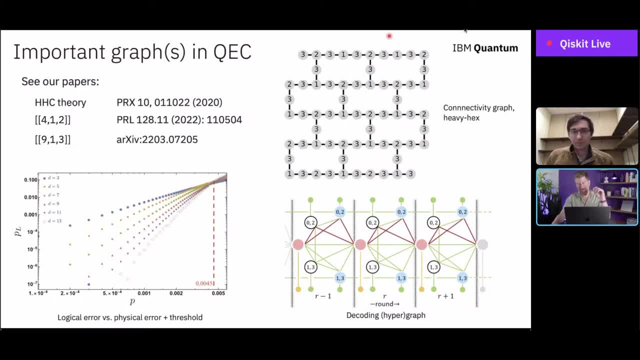 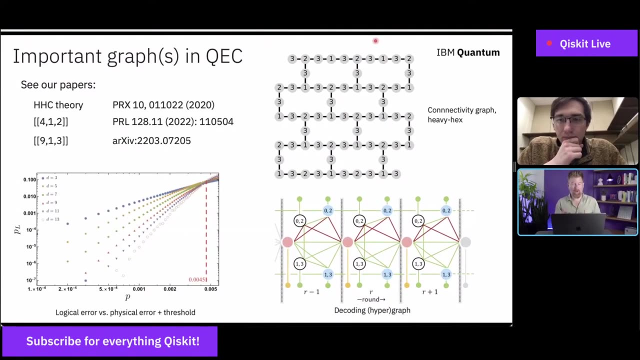 followed by my first question, which I know has been discussed, on the Qiskit seminar series before, which is certain: like radioactive events, for example, that cause the breaking of Cooper pairs can cause correlated errors across a relatively large region of a quantum processor. 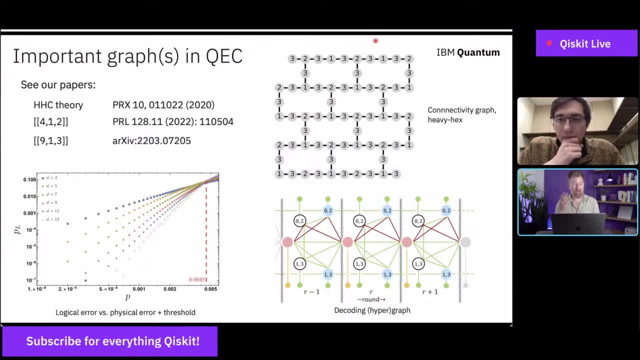 And I was wondering what kinds of codes or what kinds of research you're doing with respect to that kind of event. That's interesting. So I imagine these events are somewhat localized Exactly, And you know, geometrically local in the plane. 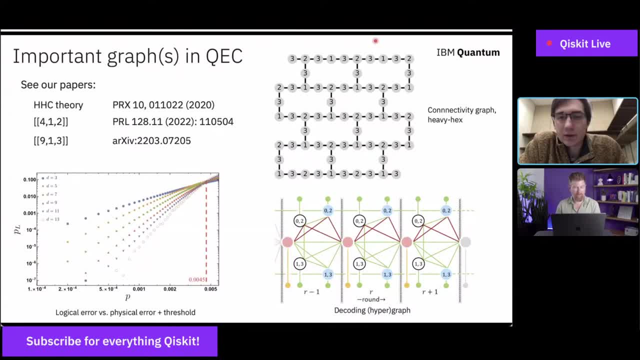 So yeah, I mean, I think the error-correcting codes that we're looking at here, like the heavy hex code or the surface code, can correct those errors, at least if the code is large enough. So here we're just looking at smallish versions. 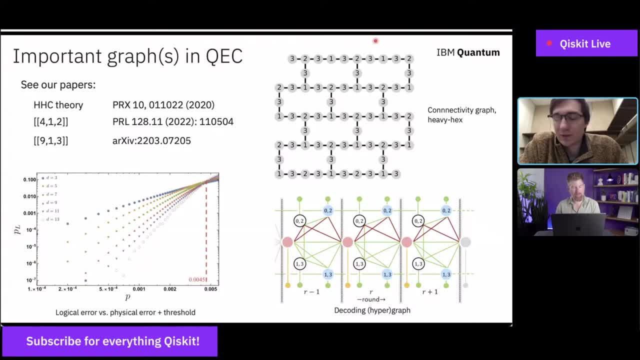 small codes and if maybe one of these events occurs and it corrupts, it'll end up corrupting a large fraction of the qubits, So it'll be uncorrectable for our small codes here. But as we scale up these might become correctable. 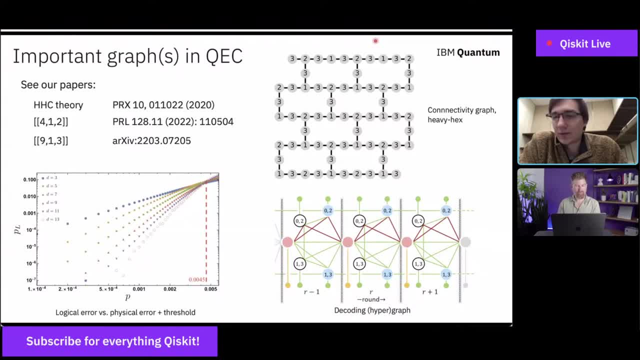 And it sort of sounds like these are more like erasure errors than maybe poly errors, But that's also something that our codes can handle, I see. So as long as the error is localized, even if it's correlated, you can still correct for it. 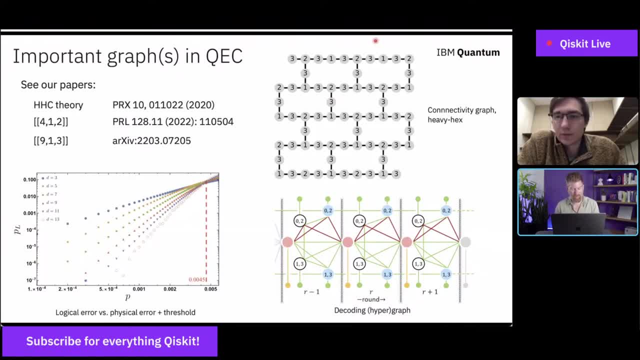 if you have a large enough code, Right? Yeah, That's good news. Let's see. There were some questions in the chat earlier, So let me see if I can ask this one: Are classical Shannon or Huffman error-correction techniques ever used in quantum? 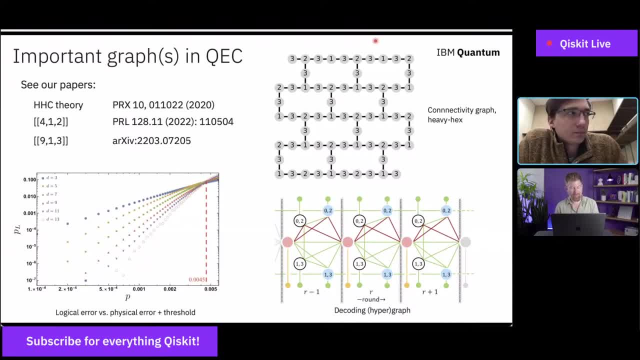 Shannon or Huffman techniques- I don't know what those are either Right. So I think Huffman coding is trying to come up with the shortest code, for I mean, as far as I know, Huffman coding is not really about correcting errors, But maybe the questioner could clarify. 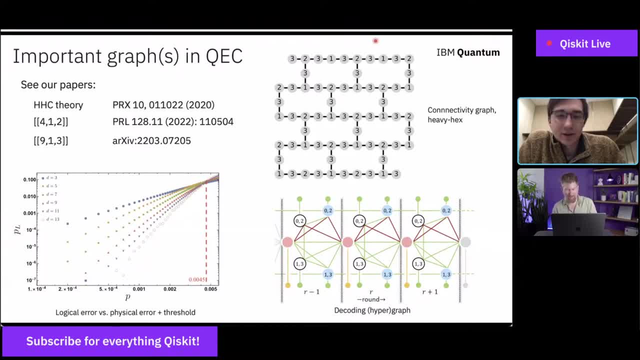 So here we're really focusing on error-correcting techniques, I think the Shannon question. So Shannon has, Or at least the theorem that you can randomly choose classical codes and they're going to be good. So quantum codes actually have some additional constraints over classical codes? 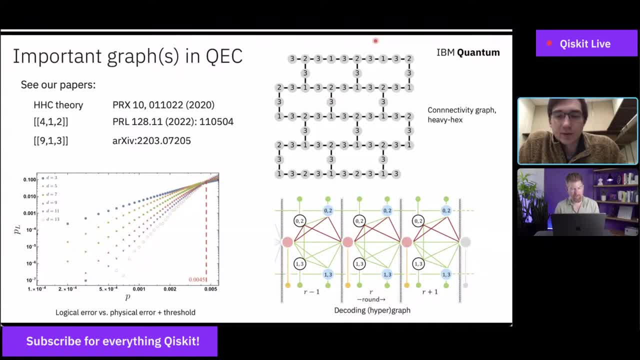 which we actually saw in our talks of the X stabilizers and the Z stabilizers, need to commute, So this actually makes the study of random quantum coding theory a bit more complicated than classical random codes. Now there are ways of taking classical codes and converting them to quantum codes. 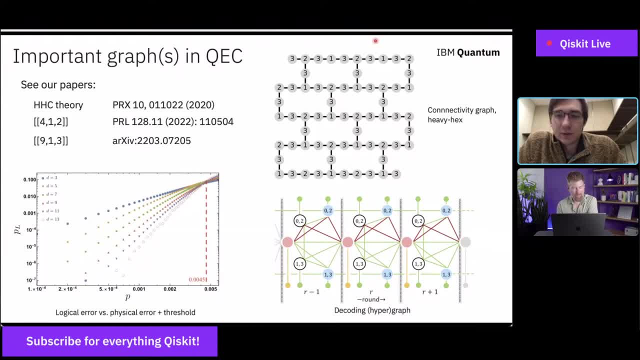 You can look at what's called the hypergraph product, And in that case you can use random classical codes and get quantum codes that are, They do, somewhat decently Cool. OK, here's another one from the chat. Oh, I got a. 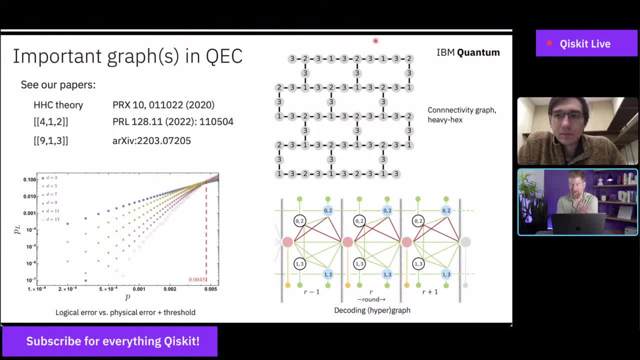 Yes, Huffman codes are more about compression of information than correction of actual errors. So confirmation from the chat. There was another one I kind of answered in the chat because I kind of use Pulse a lot. But the question is, is there a best way to learn? 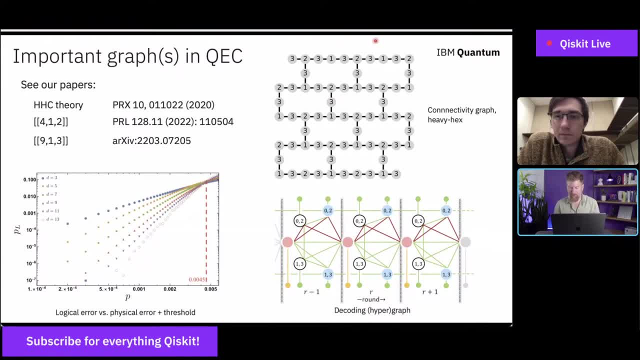 how to do error correction codes work using Pulse, or would it be better? Yeah, that's basically the question. My thought initially was, as far as this is all about Clifford circuits, basically just using Pulse to tune up the best Clifford gates is what's important here. 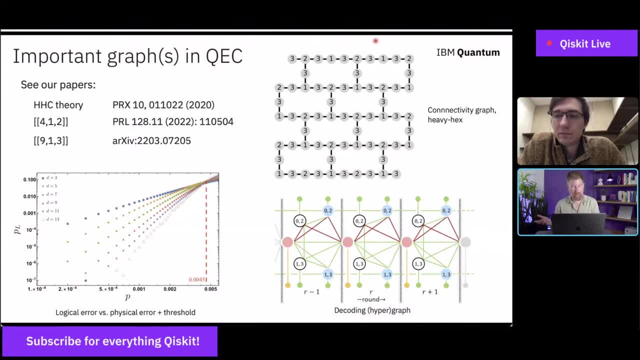 But then I know we've had other chats about driven dissipative systems or control, like a Floquet qubits for example. It's kind of adjacent, not exactly the same kind of error correction work, But I was just wondering if you had any thoughts on that. Right, So something I- I mean this is sort of This is adjacent to the question- Something I didn't get to here was that we actually do some like dynamical decoupling as our, as our parity checks are happening, So sometimes there are qubits. 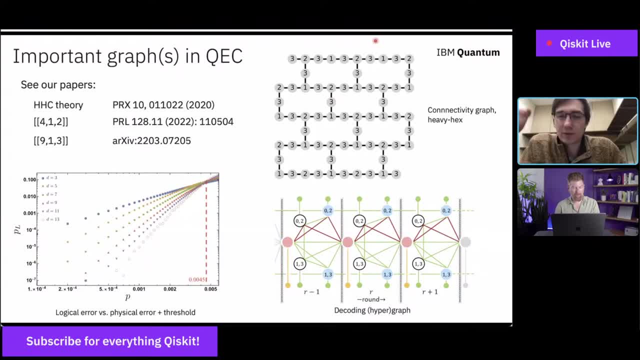 that are just idling, And so we do dynamical decoupling sequences on those to suppress Z errors that might occur. And this actually makes a pretty big difference for the logical plus and minus states which are sensitive to these Z errors. Yeah, 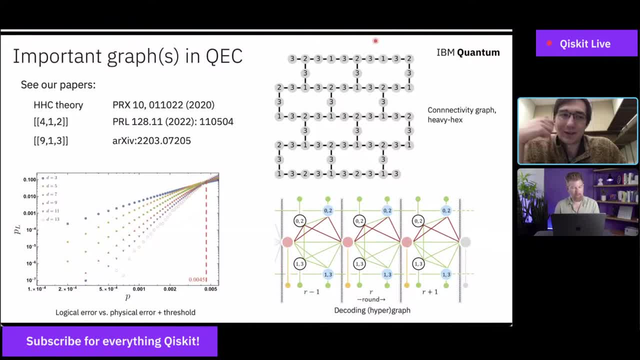 I mean tuning up gates and doing certain pulse sequences to suppress errors is actually an important compliment to these error correcting codes. Absolutely, Error mitigation seems to be a very hot field in the noisy near-term error of quantum hardware before we get to the kind of thresholds. 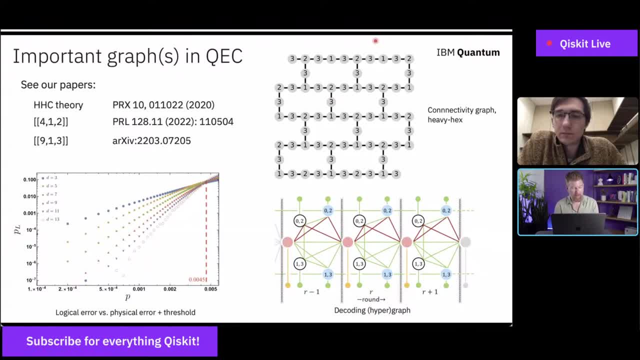 where we can reasonably do logical encodings, for example. And so you kind of entertained. my last question, or my last question is: is there any kind of like hybrid, kind of like maybe I want to say like partial error correction, Like would it be useful? 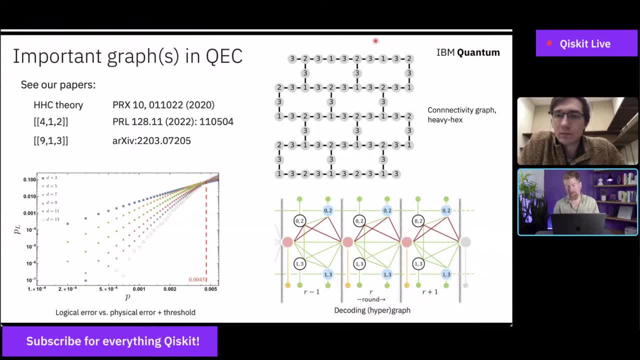 in certain algorithms to try and error correct, say, idling qubits- I'm just thinking of an example- or any class of qubits in an algorithm that could be, you know, somewhat corrected to get an advantage over not doing any correction. 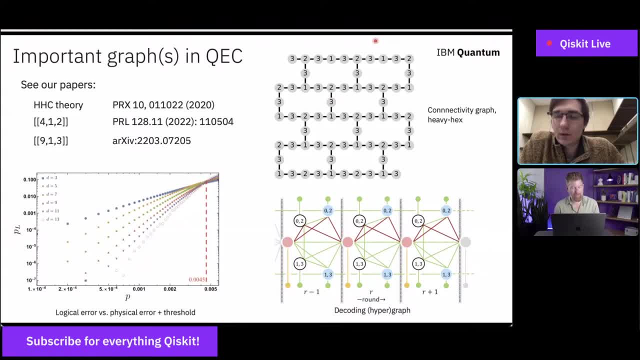 Yeah, So I think this is getting to like open questions in the field. I mean, it depends on your algorithm, And probably the type of error matters here as well. So I mean you can imagine that X errors are more problematic. 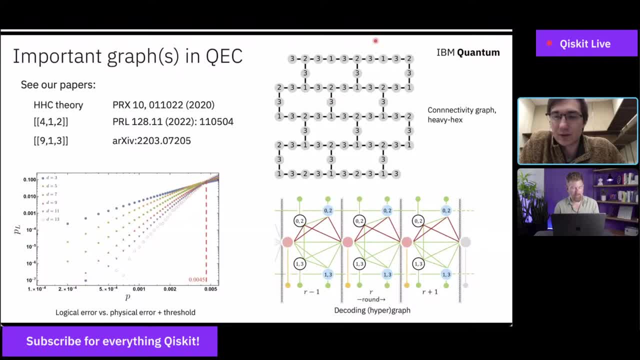 at some points in the circuit than Z errors, Like if you're just before you're measuring out the information, then you don't actually care about Z errors, Right? So quantum error correction: it can be used to suppress just one type of error. 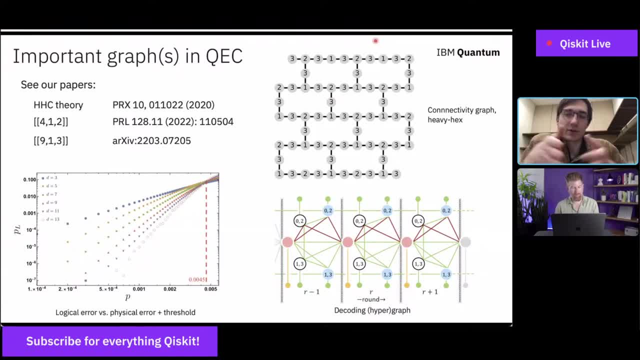 and leave the other. So if you make like the surface code, asymmetric, say you like, make it a rectangular code instead, or you could do the same with the heavy hacks. then you can preferentially suppress one type of error. 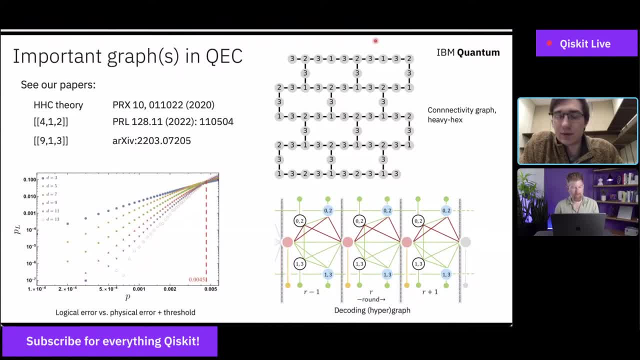 and leave the other. I think you also brought up error mitigation, And so you could imagine using error correction to suppress errors to some extent and then using error mitigation on top of that to suppress it the rest of the way, And maybe that's cheaper. in terms of qubit cost, because the full-blown error correction would require a lot of qubits, a large patch of surface code, But then the error mitigation just repeats the same circuit on the same patch of qubits, on the same smaller patch. 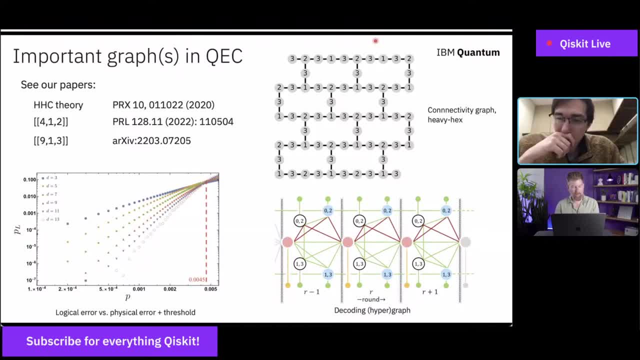 And so you can use that to get the rest of the way. Yeah, exactly, I think, alluding to kinds of areas of exploration that will be really important in these kinds of larger qubit, lower error kind of place between the noisy and the error corrected. 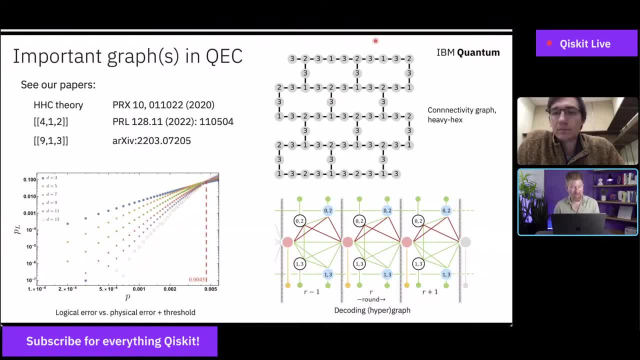 where I think. personally, I believe there's a lot of room for exploration in these areas, So I think that's very interesting. Yeah, we're definitely just in the early stages of experimental quantum error correction. right, These are the smallest codes. 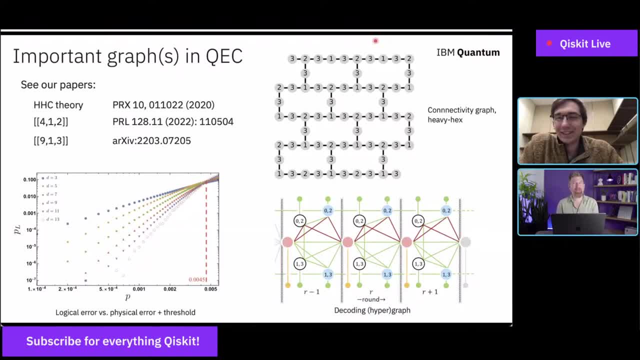 that you can possibly implement, Exactly As you can see in the little tutorial we put out today as well. Yeah, It seems like I think that's all the questions that we have today. I want to thank you so much for that wonderful talk, Ted. 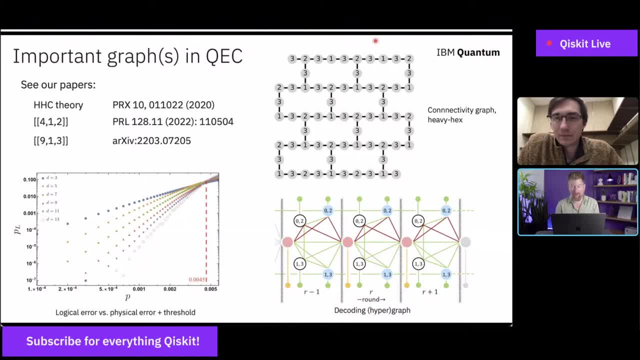 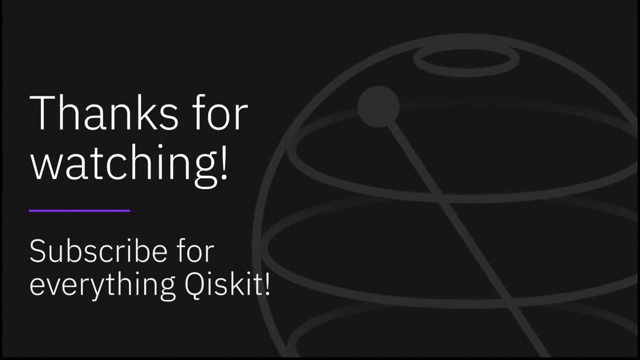 And it's great to talk with you again, And I encourage our viewers to like and subscribe to Qiskit YouTube and we'll see you next week. Thanks a lot, Nick, Take care Bye.